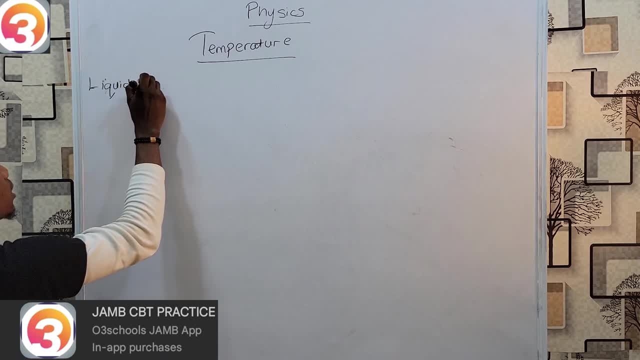 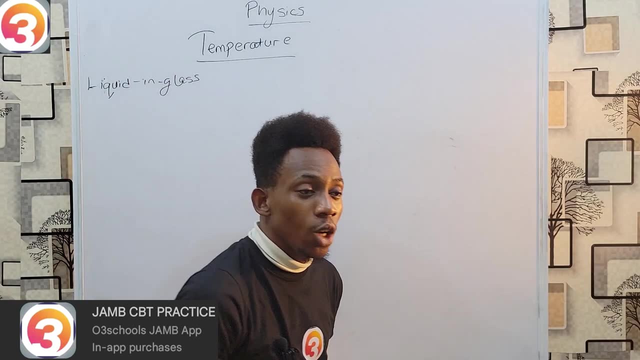 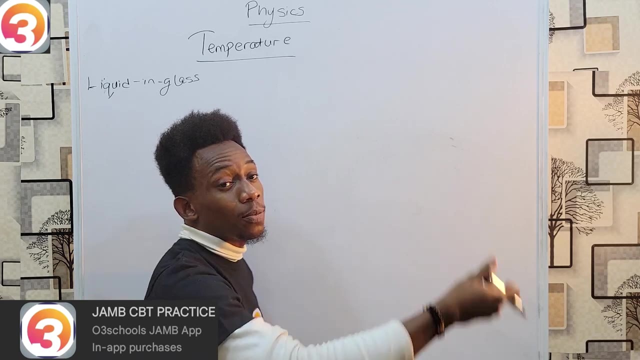 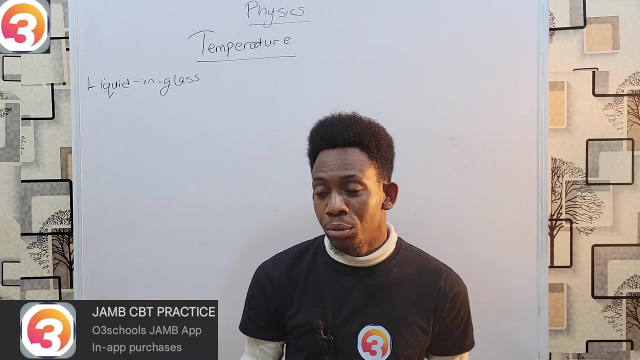 That's liquid in glass thermometer. This liquid in glass thermometer measures the change in the volume of a liquid with temperature. So all you simply have inside is a liquid, and as temperature changes this liquid expands. Now every thermometer that has a certain material would survive always changing in temperature such that they can sense it when 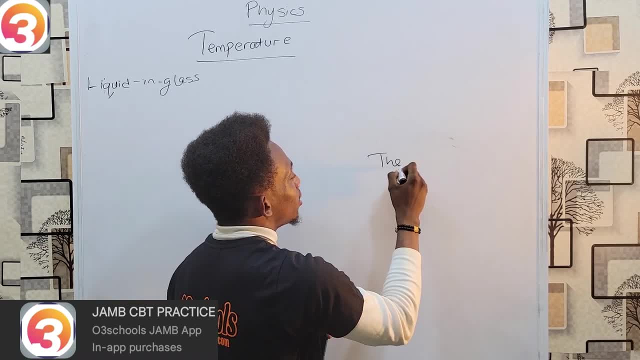 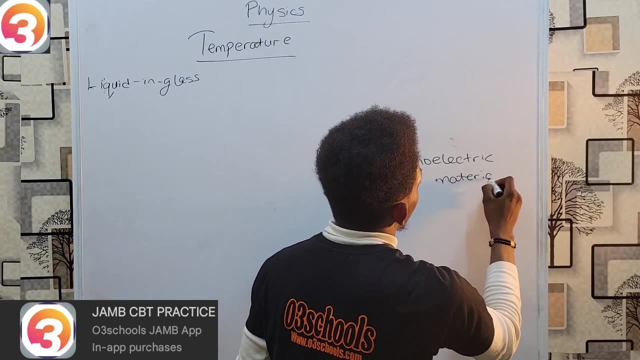 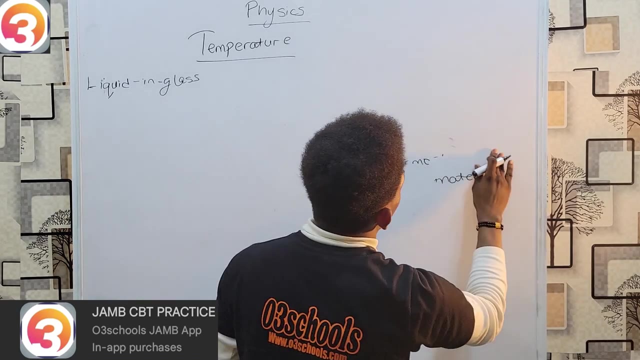 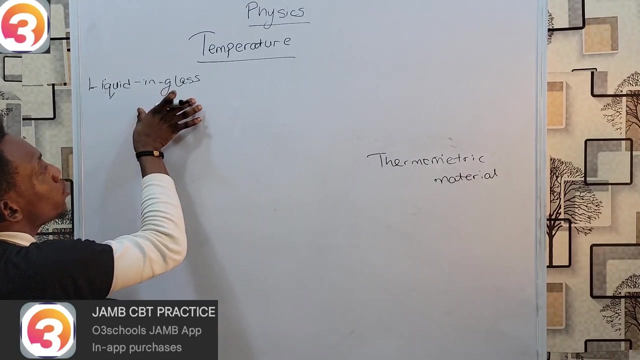 temperature changes. This is a material referred to as a thermoelectric material, a thermoelectric material and in this case automatic, a material for- sorry, not the military- thermometric thermometric, do not mind me- thermometric material and the thermometric material for liquid in glass. thermometer is really either alcohol or mercury. 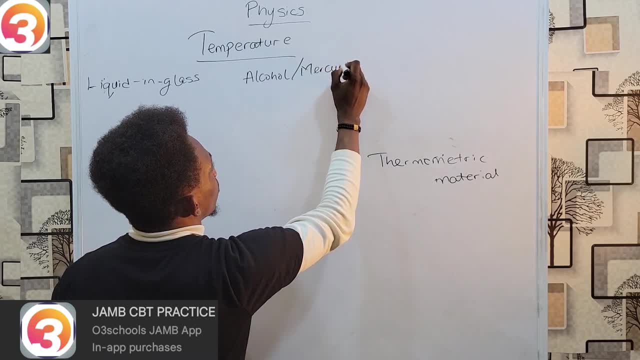 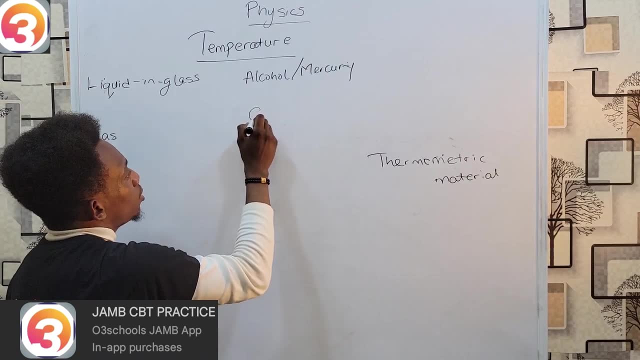 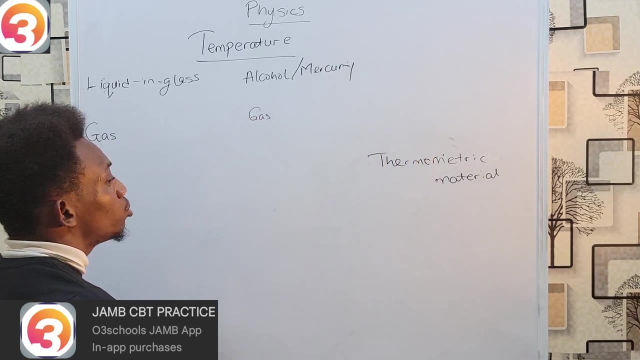 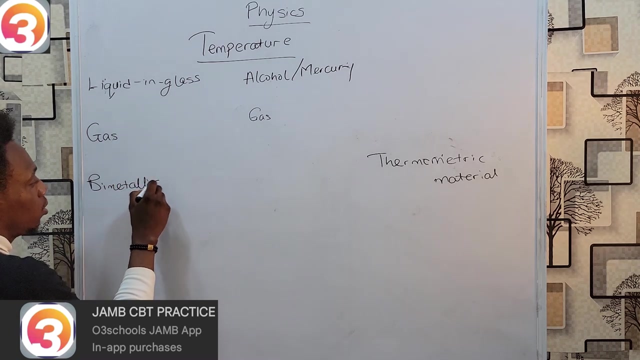 on that liquid in glass. we also have gas thermometers. gas parameters simply make use of any gas and they measure the change in the pressure of this gas at constant volume. there are others, so you have your biometallic strip, you also have thermocouple and you also have 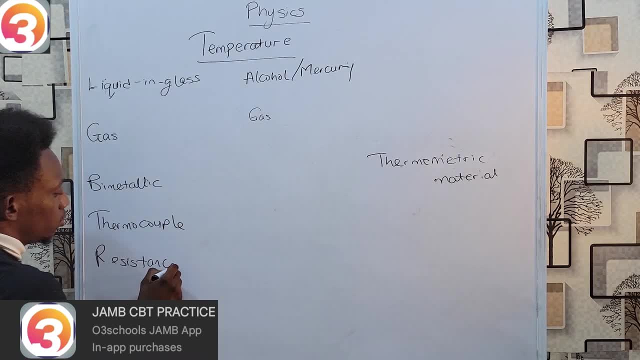 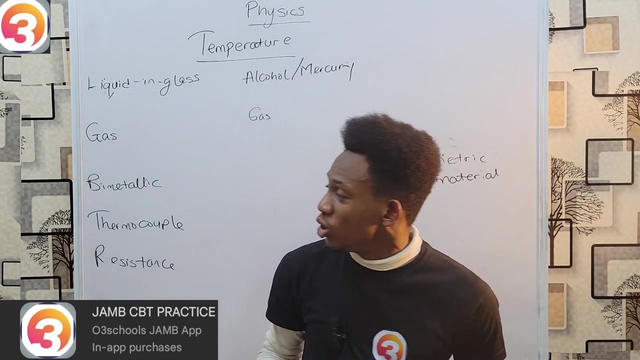 resistance thermometer. resistance thermometer measures the change in resistance with temperature. uh multiple couple measures the change in potential difference with the junction between two dissimilar metals, while the metallic thermometers measure temperatures due to the difference in expansion of two dissimilar metals. so these are types of thermometers. however, in the 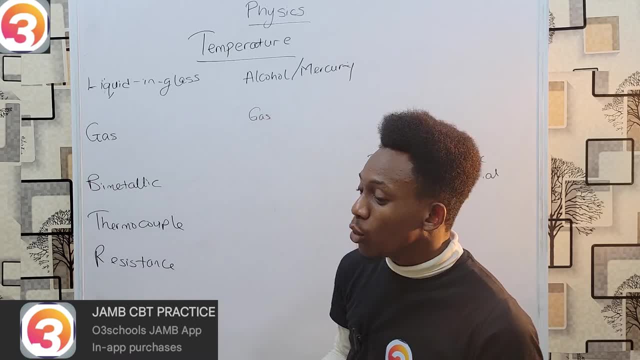 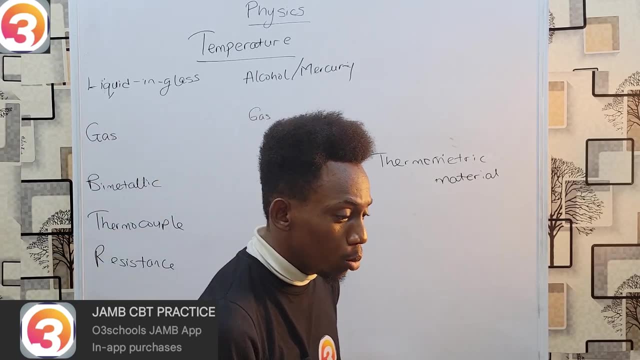 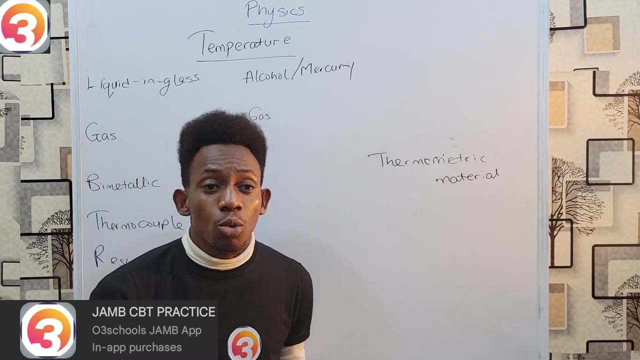 course of the syllabus, we are made to focus more on the liquid in glass thermometer. now, looking at the glass thermometer is quite special. like we said, mixes of either alcohol or mercury. however, i may say what are the qualities that makes me know this thermometer is making use of a good thermometric material? 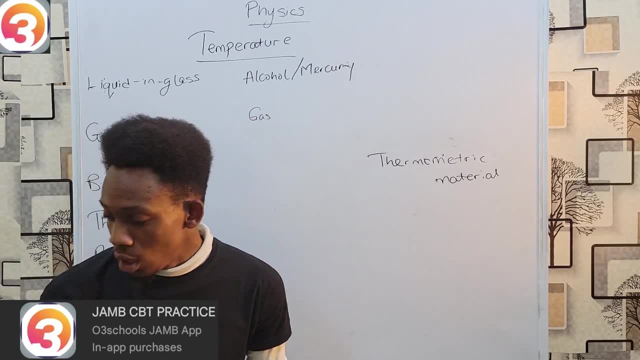 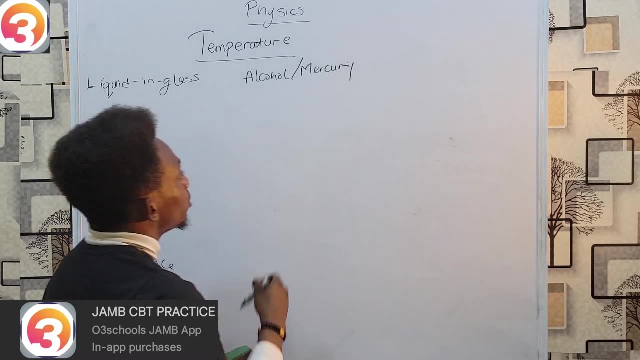 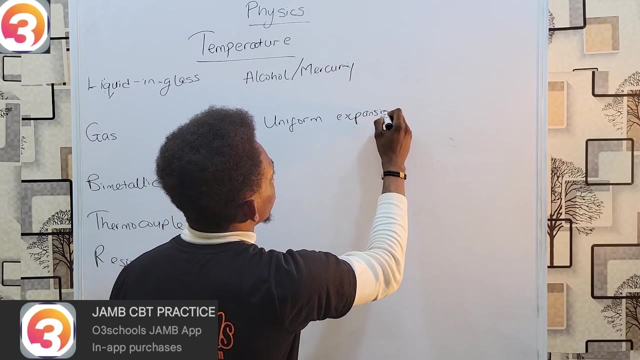 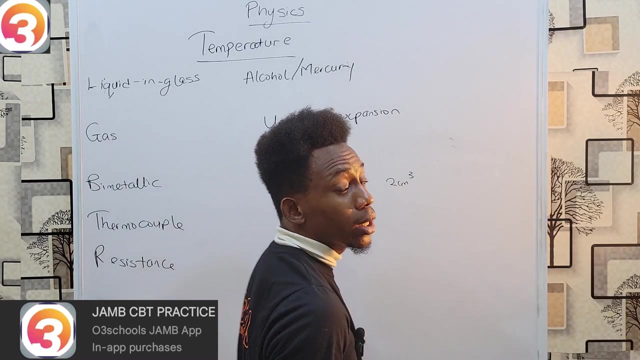 or in this case, it is really a thermometric liquid. now, one of the important things to look out for in making our decision that this material must have a uniform expansion. that means the expansion as temperature changes also be uniform. it could increase by maybe two centimeter cube for every degree rising temperature. that will be constant. 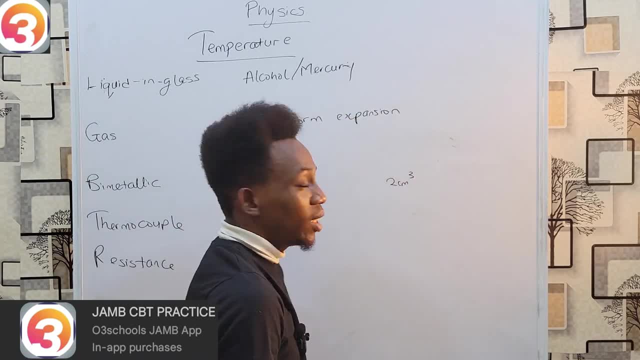 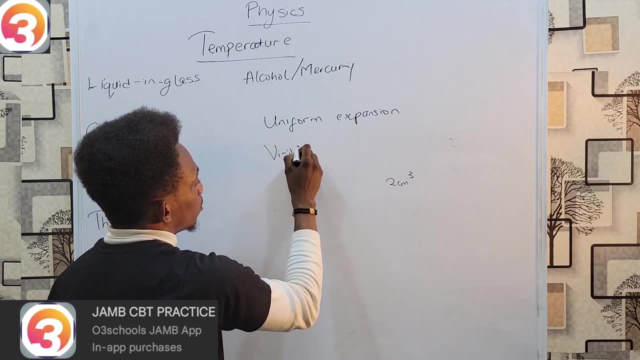 that would be uniform, making it easy for us to calibrate this thermometer. then also, a good thermometric liquid must be visible through the glass, must be visible through the glass. that means i should be able to calibrate this thermometer. that means i should be able to calibrate this thermometer. 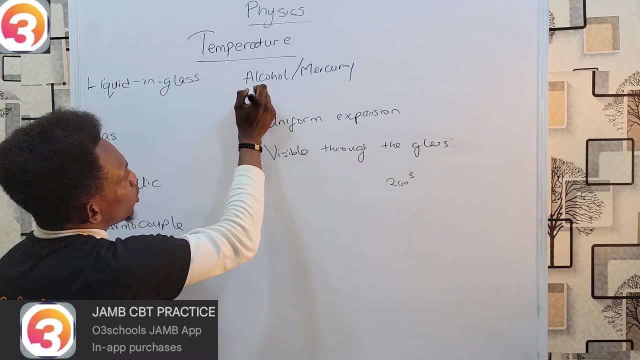 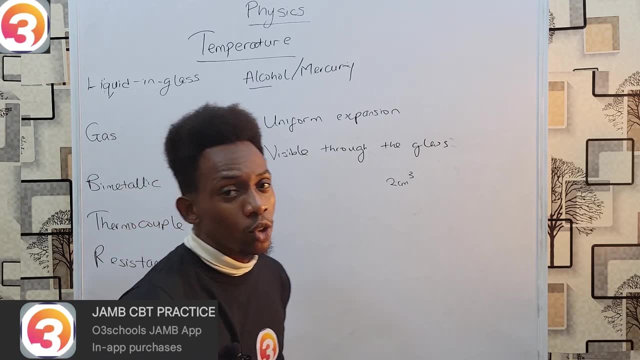 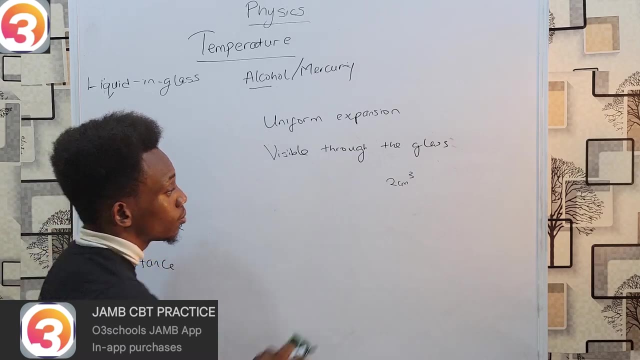 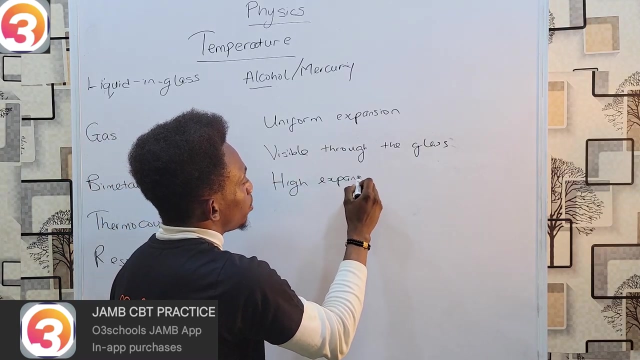 to see it easily. now, alcohol has a little bit of a defective. alcohol is rather translucent, but for that reason a bit of coloring is very added. to make alcohol suitable- because its other advantages will outweigh this slight disadvantage, then it must also have high expansivity. now what this implies is that if my thermometric liquid doesn't expand sufficient, 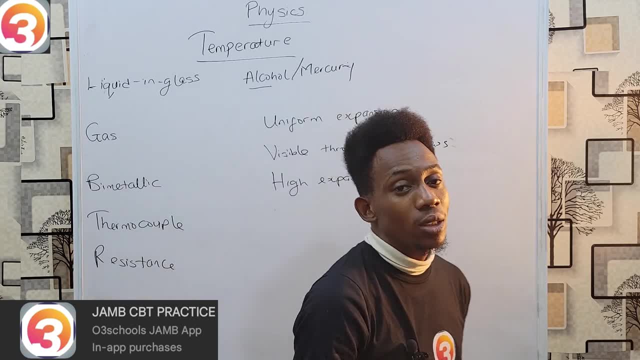 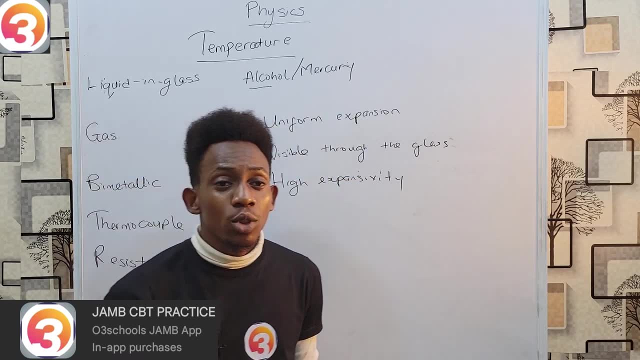 with the change in temperature, then i won't be able to actually measure anything. if this, if this liquid has to maybe undergo a change of 10 degrees celsius before any noticeable change occurs, my thermometer becomes rather useless, because i'm able to measure any change going on between that one to nine, until it gets to ten. so it must have high expansivity. 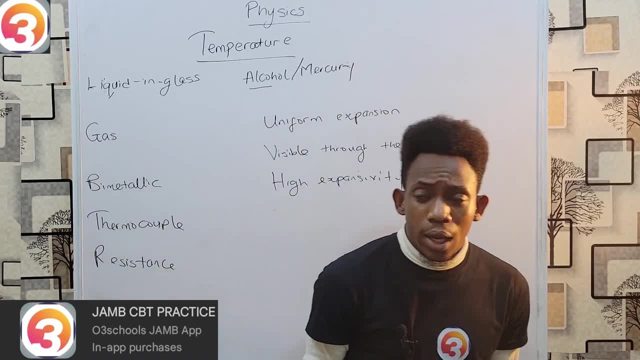 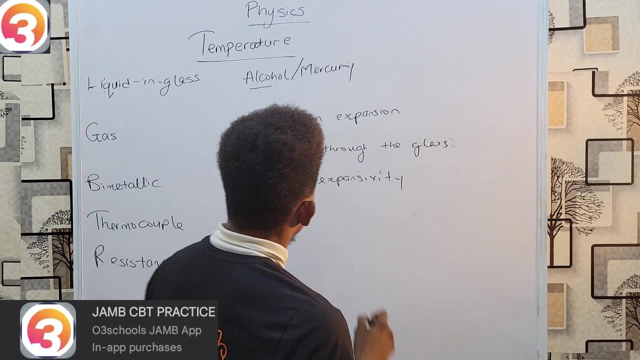 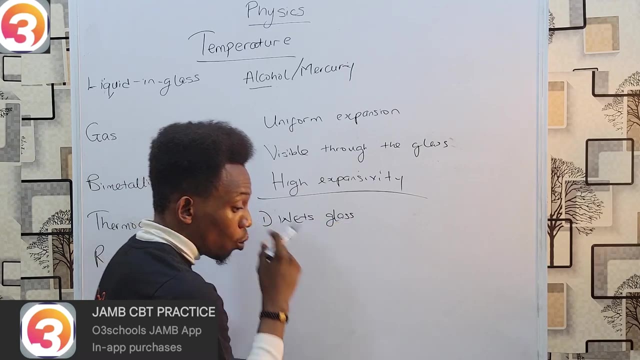 now that there is also the question if i'm using a liquid, as a human, our first thought is always water. so if i'm using a liquid, why not water? well, first of all, one is because water wets glass. therefore, water wouldn't work quite fine for a thermometer. 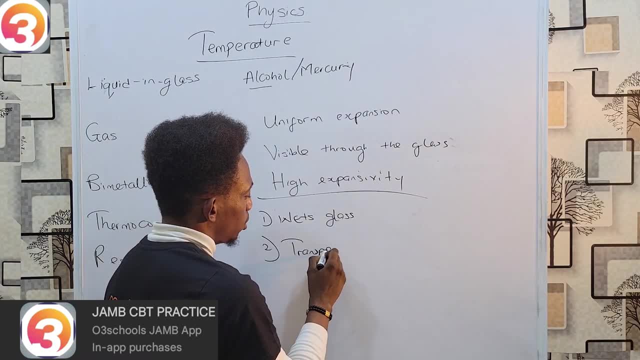 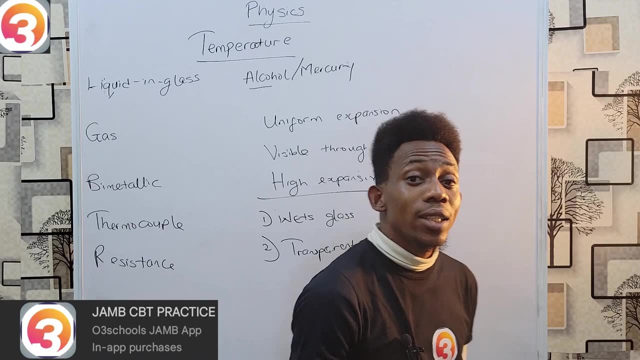 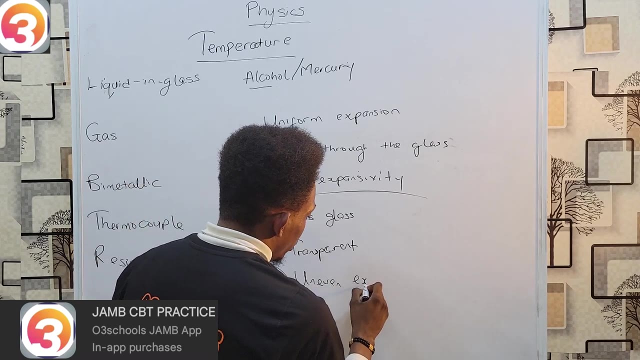 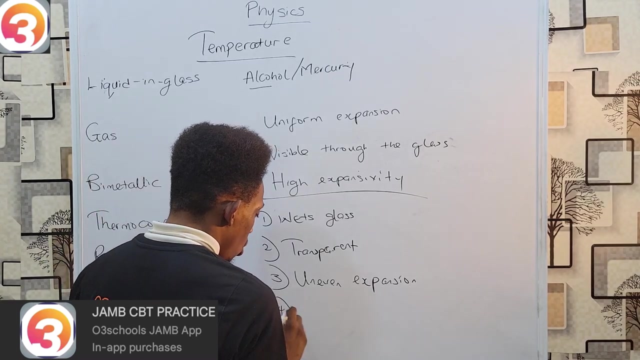 two: water is also transparent, that is colorless, so we can see through water, which makes it rather difficult to use in a thermometer. and then also water doesn't undergo even expansion, and in this case we refer to the animalous expansion of water. then also, water has a high freezing point. 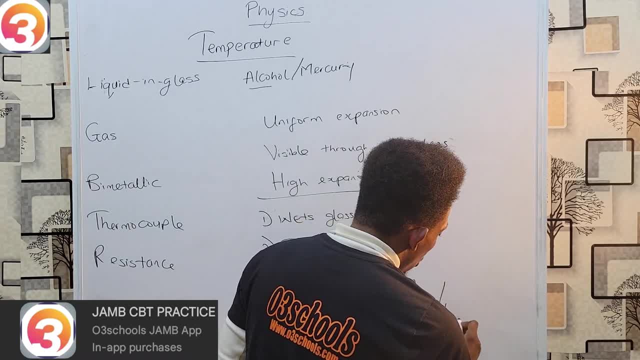 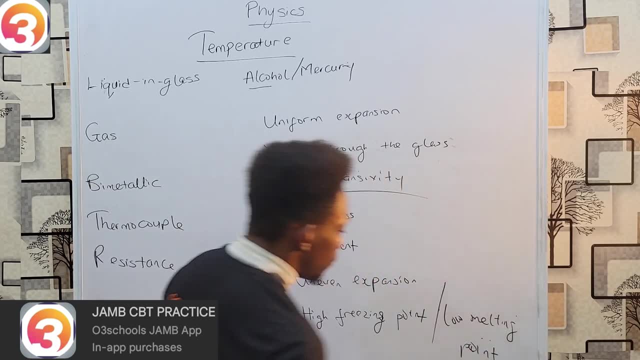 and a low melting point. sorry for obstructing you just a bit here. high freezing point and a little melting points. what this indicates is that the high freezing point is at its lowest point in the temperature you're dealing with. so even a little bit higher freezing point can cause water to be destroyed by THAT HIGH FRIZING POINT. 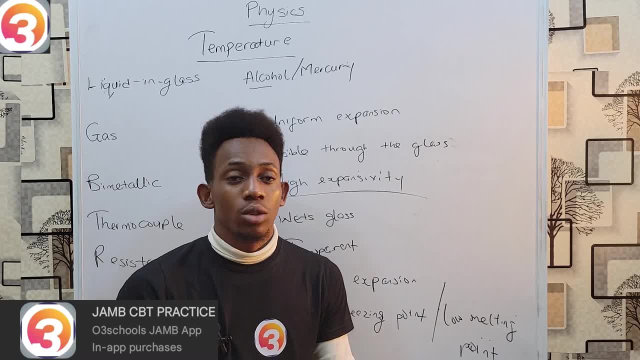 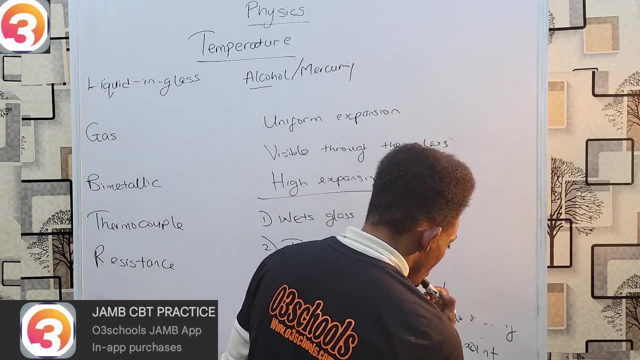 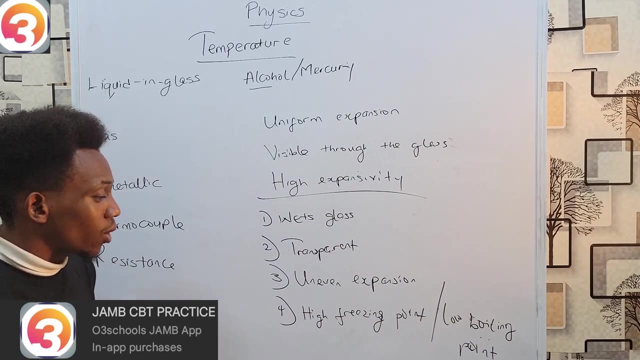 and a low melting point can cause water to be destroyed by THAT HIGH FRIZING POINT. As you are aware, under standard pressure, water freezes at 0°C and boils at 100°C. As a result of that, it means that once you measure anything below zero, instead of having 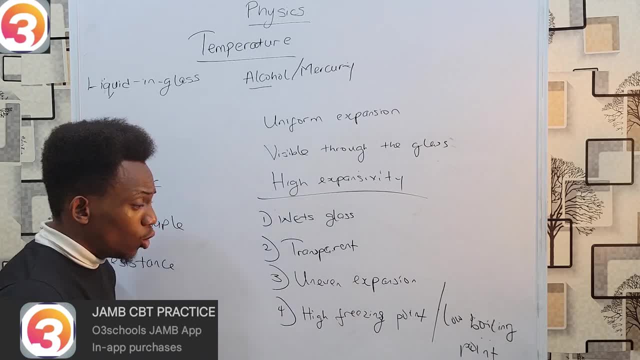 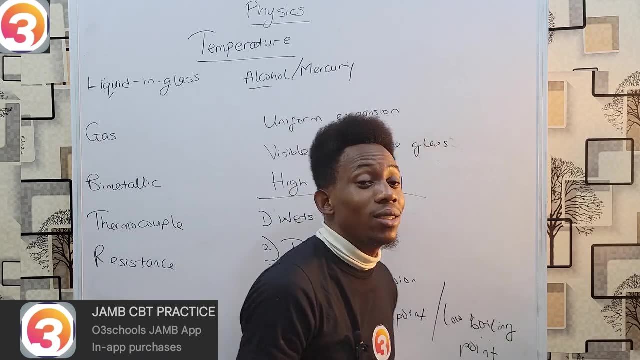 a liquid in glass, you'll be having solid in your thermometer, which makes it automatically useless, And once you're trying to measure anything above 100°C, you'll then be having gas in your thermometer, which makes it again useless for a liquid in glass thermometer. 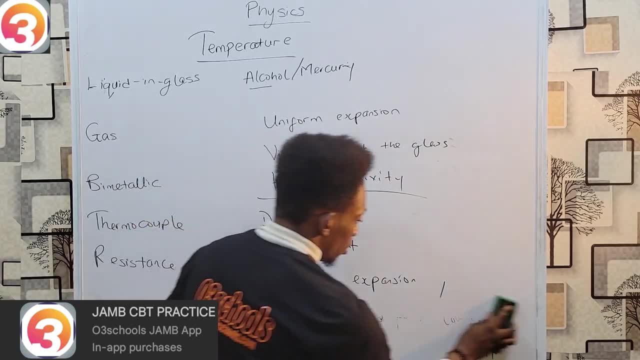 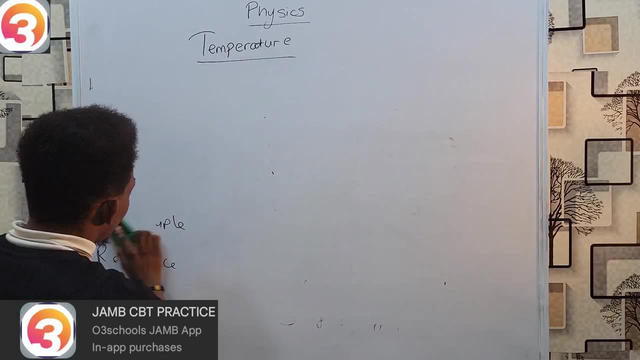 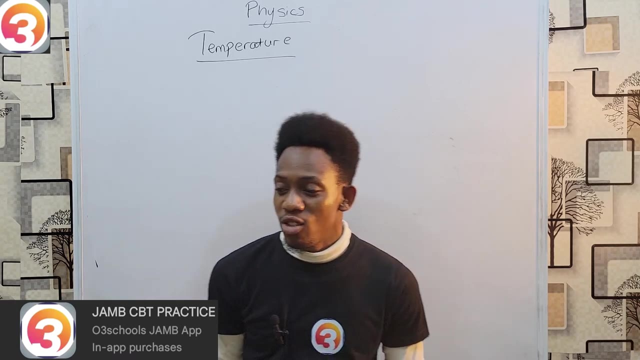 And for that reason we do not use water. Now, on deciding what type of thermometer you are going to use, before making your choice, knowing you'll not use water, you also have to decide, okay, where do I use alcohol And where do I use mercury, Or can I just use them nilly-willy? 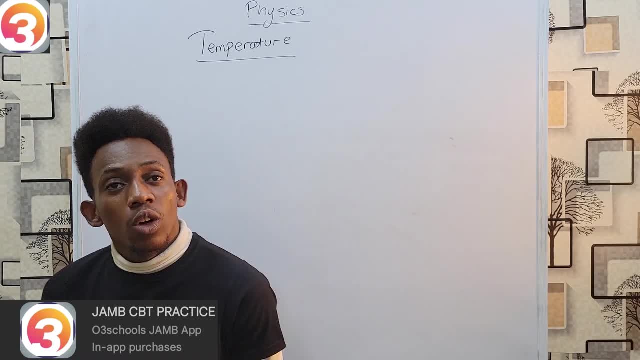 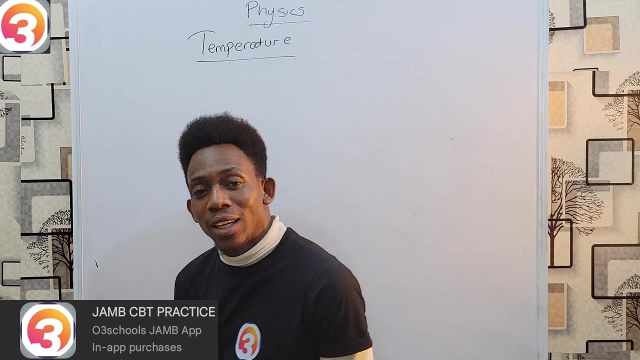 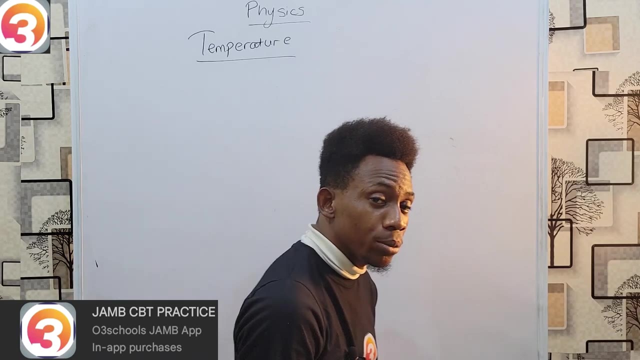 The question then becomes to decide. you must ask yourself, while I'm measuring, how high is the temperature or how low? Mercury has a rather high freezing point. Therefore, it's easy for mercury to turn into a solid. So do not use mercury to measure very low temperatures. 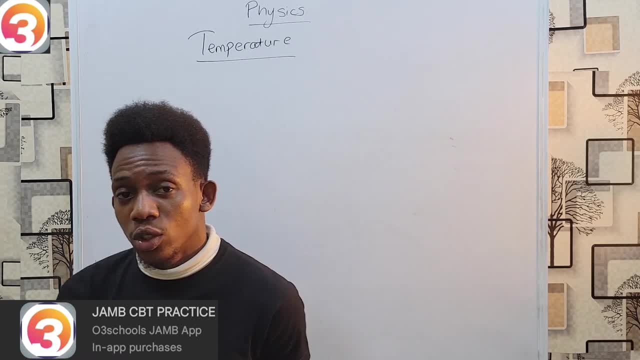 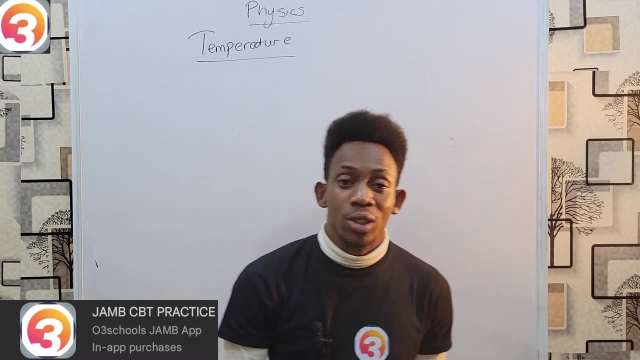 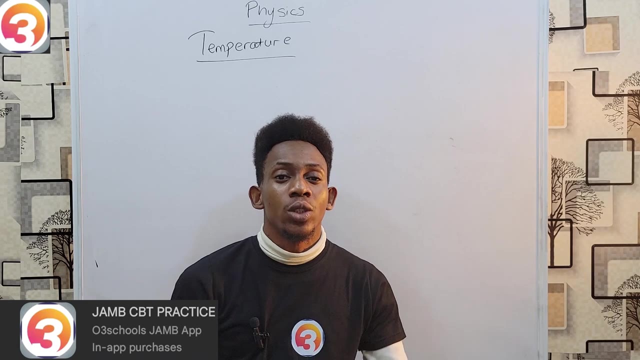 but alcohol can be used to measure low temperatures. On the other hand, alcohol can boil rather easily, So do not use it to measure high temperatures, while mercury can be used to measure those high temperatures. And so far we've been talking about measuring this temperature and measuring this temperature. 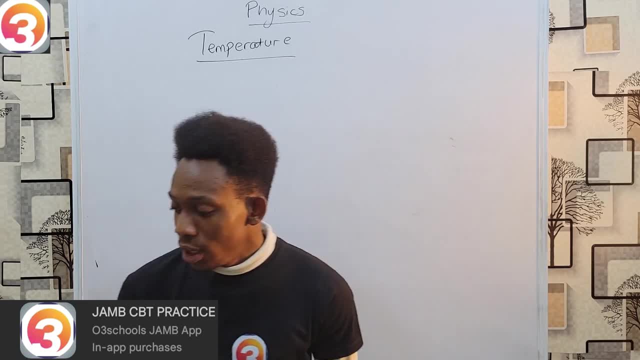 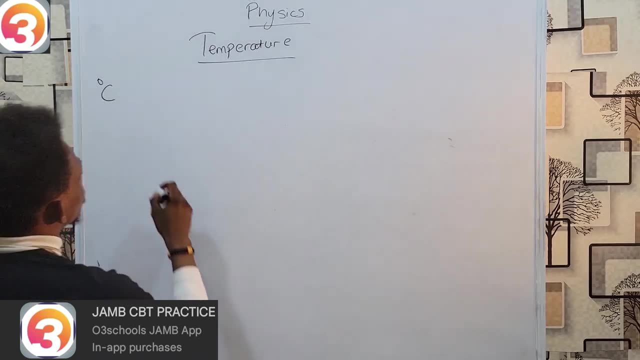 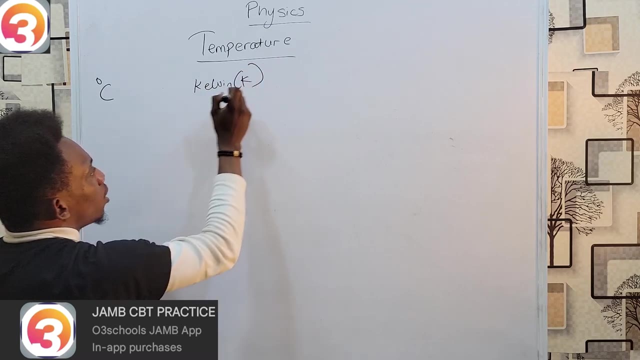 Where do we measure this temperature? What is our unit? Now, as a Nigerian, the common unit to be aware of is degree Celsius, But, as you should be aware, the S-sinus for temperature is Kelvin K. K also known as the absolute scale of temperature, absolute scale. so, in this, 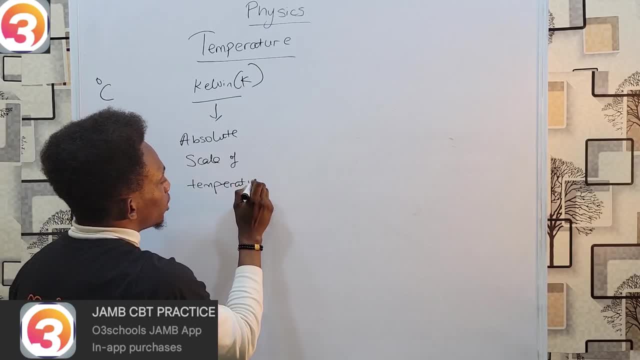 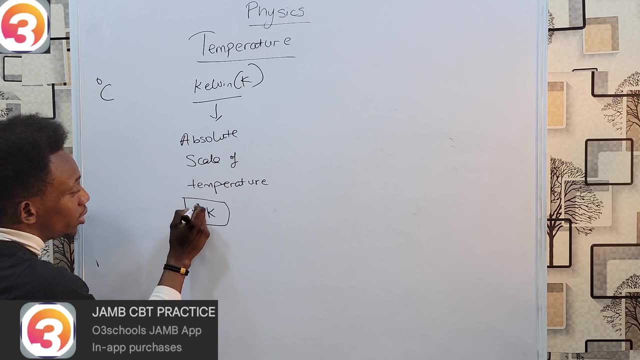 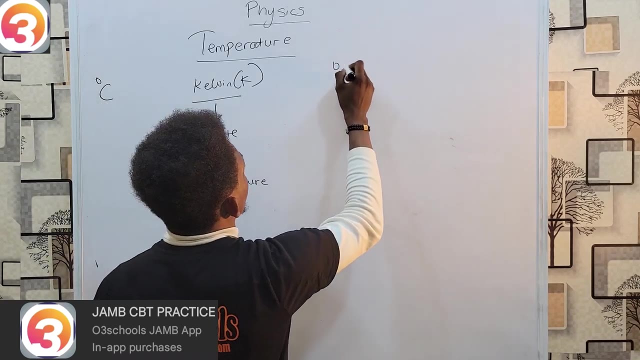 topic. you'll notice that the lowest value that the material can freeze to is zero Kelvin. this is not okay. this is zero Kelvin. that is the lowest value. Kelvin is absolute scale. then we also have under scale, which is your Fahrenheit scale. then there are a few others, but these are the most common ones to look at. 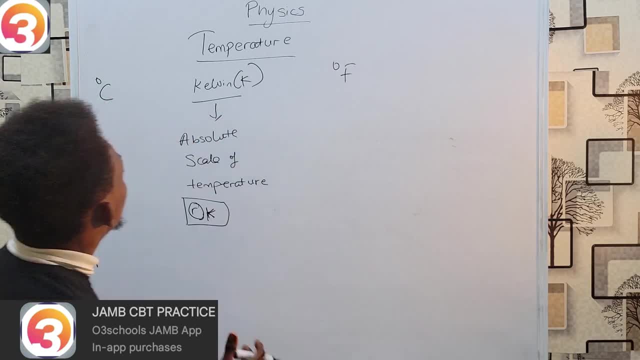 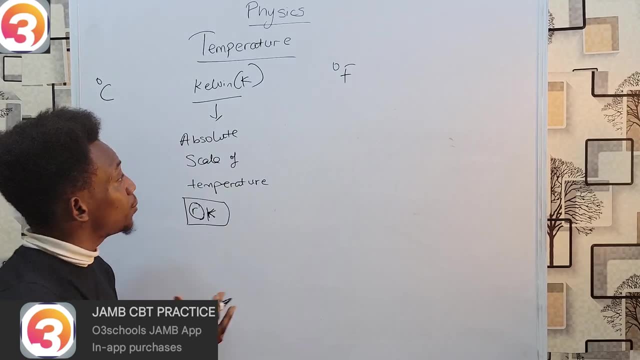 there's also Rankine, but we will not deal with that at this level. we focus purely on degrees Celsius, Kelvin and Fahrenheit. now, when using these different things, if you have to convert from one to the other, how do you go through with your conversion? all you have to look at when trying to convert is: we have two things. we look at number. 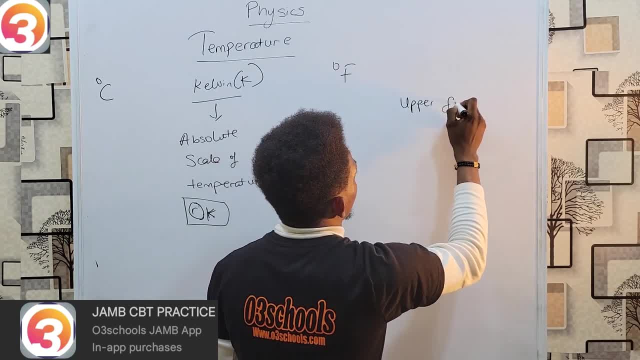 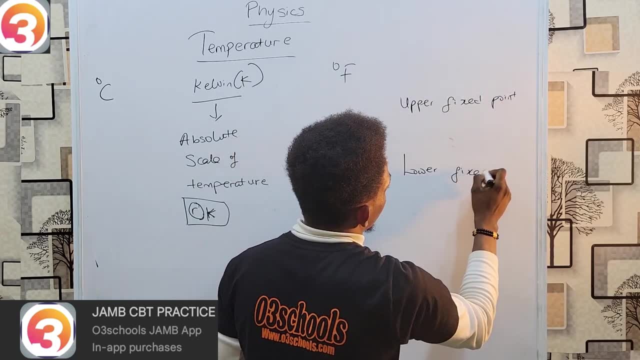 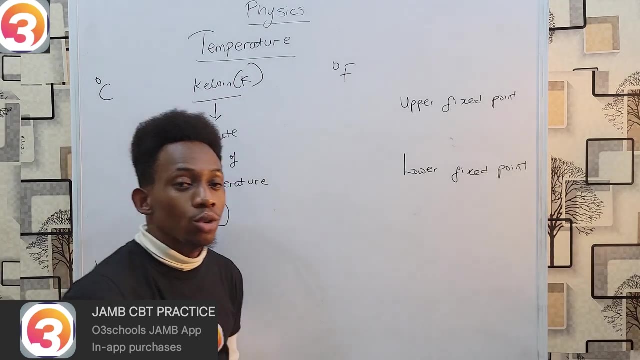 one is the open scale fixed points- upper fixed points- and the second is the lower fixed points. now what we'll say is: what do we mean? the upper fixed point is the temperature at which pure water boils under standard pressure, while the lower fixed point is the temperature. 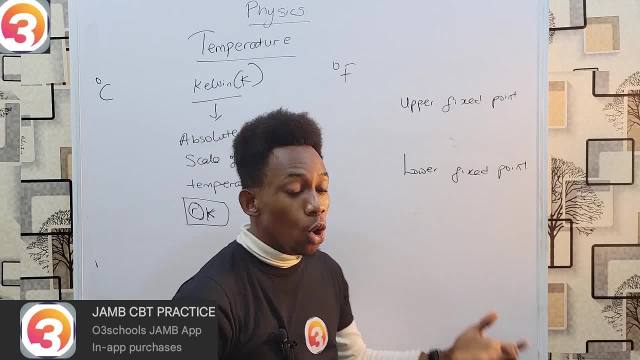 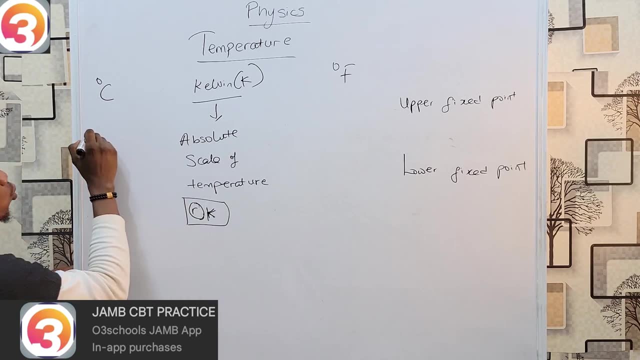 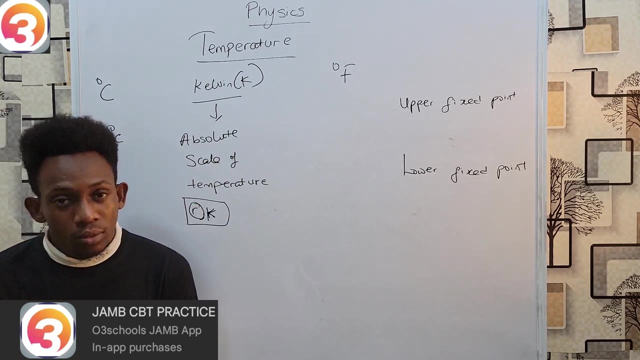 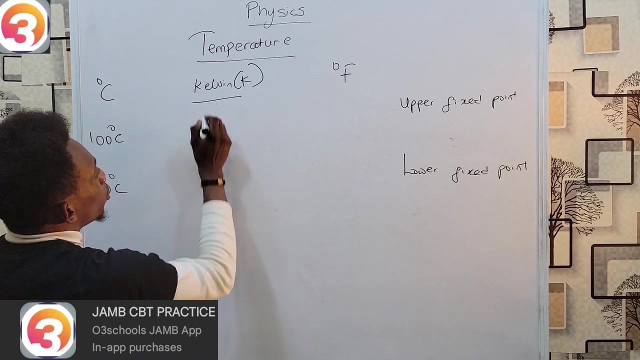 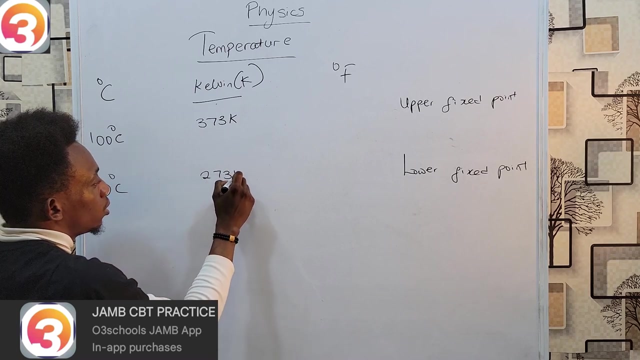 at which pure ice melts at also standard pressure. now um, commonly we must have this in primary school- pure water boils at 100 degrees Celsius, while it freezes at zero degrees Celsius. but if we take a look at our Kelvin scale, it is not the same value. in Kelvin scale, pure water boils at 373 Kelvin and freezes at 273 Kelvin. 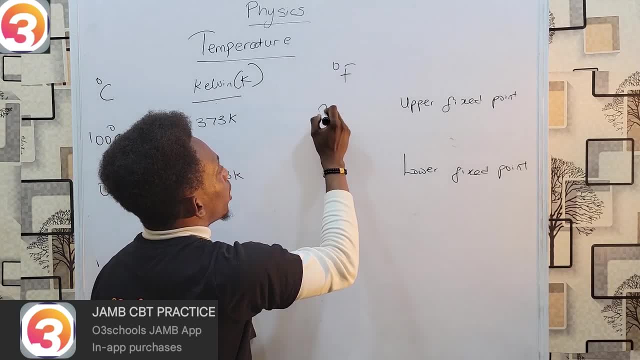 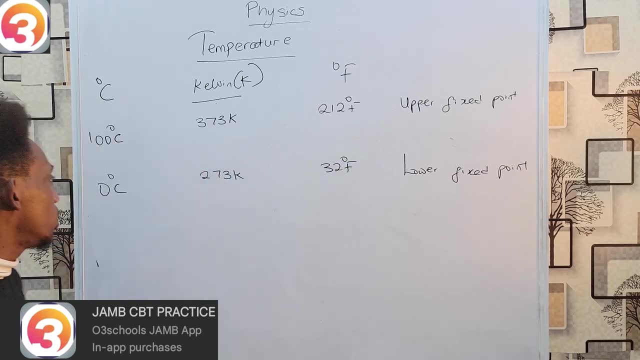 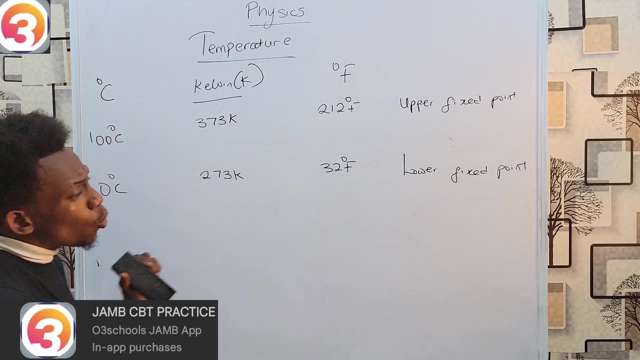 then in degree Fahrenheit, pure water boils at 212 degree Fahrenheit and freezes at 32 degrees Fahrenheit. now these values ought to be committed to memory, because in questions we have to apply them. there's also one more thing, not as important, but we should probably know it as well. it is known as the fundamental interval. 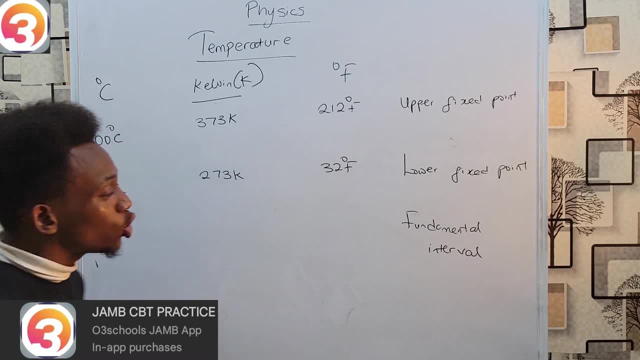 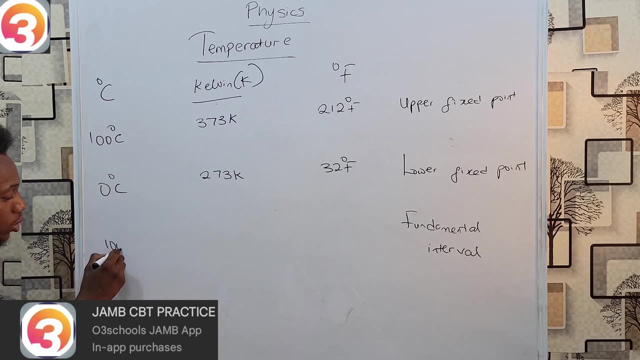 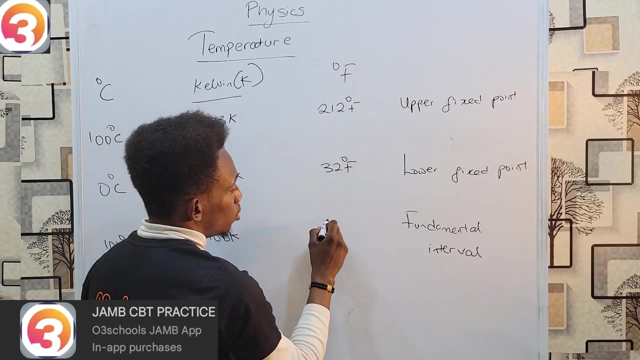 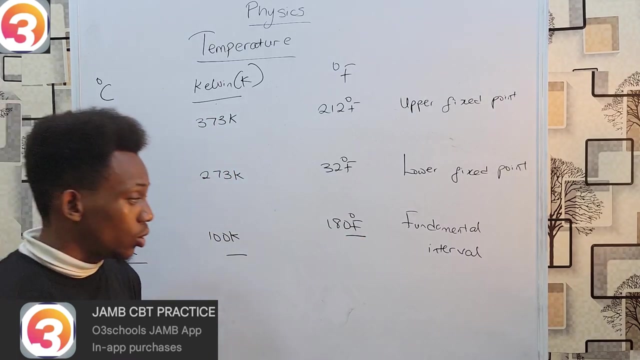 this interval is simply what you get when you subtract these temperatures. for example, upper minus 0 is 100 degrees Celsius, 373 minus 273 is 100 Kelvin and 212 minus 32 is 180 degrees Fahrenheit. so these are the fundamental intervals and um when combating from Celsius to Kelvin, there's a rather simple method for doing. 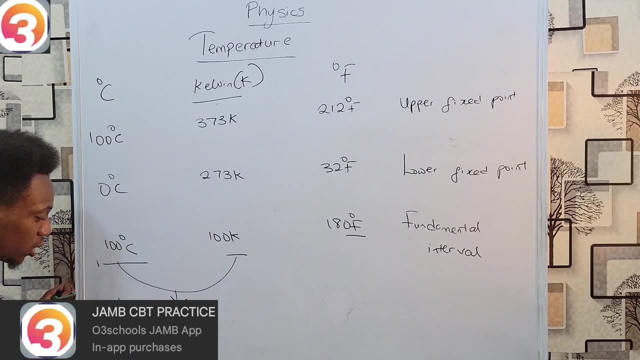 that to get a value in Kelvin, simply take the value in Celsius and add 273 to it. it's that simple. if I'm going from Celsius to Kelvin, or rather from Kelvin to Celsius, take the value in Kelvin and subtract 273.. so, as you can see, this one is very, very simple. 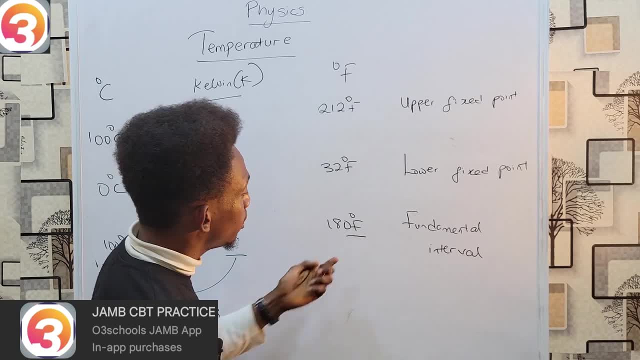 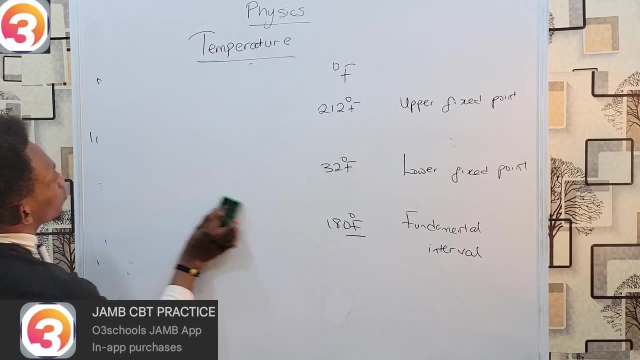 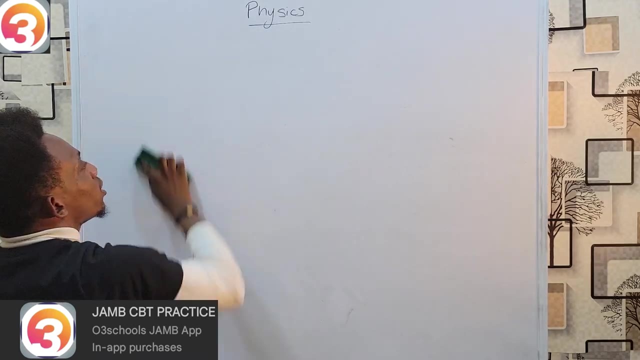 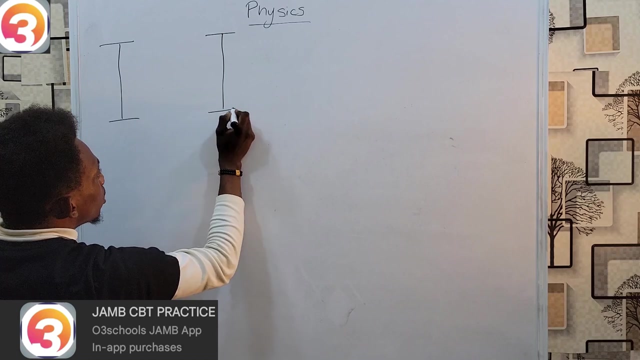 um, we could also generate a formula for doing that in Fahrenheit, but, um, while creating the formula, which I have to observe, the general method for converting any temperature skill. now, if you have any temperature scale to combat what you simply do, all you have to do is draw something like this. it doesn't have to be very big any's, as we do now. 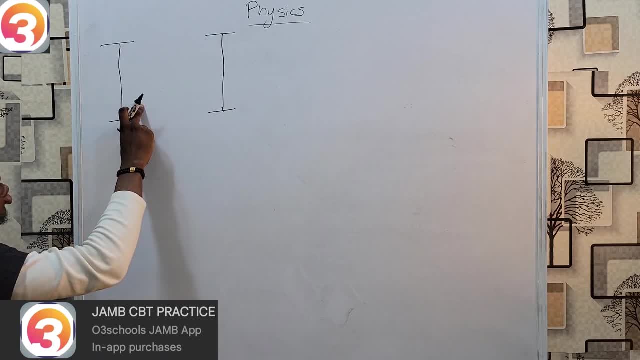 so расскcity to me is all you have to do forprés. we shall place the upperéta fromaj, unknown to qри intensitivity, to the international temperatures. place the upper fist points and at the bottom the lower fist points. so say i'm. 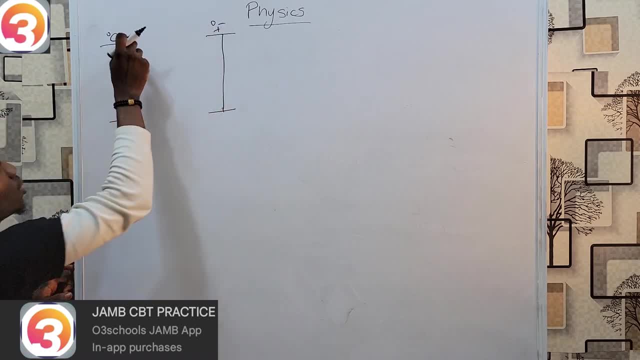 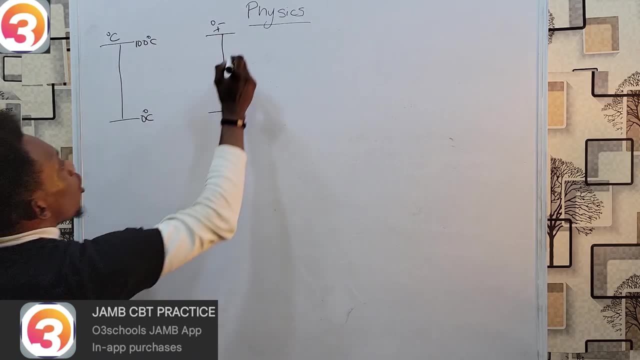 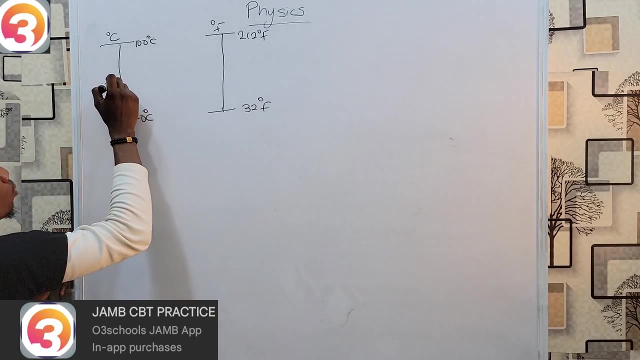 comparing from celsius to fahrenheit and the top here upper must be 100 and lower must be zero, while in fahrenheit upper must be 212 and the lower must be 32. so say, i want to convert any value c to a corresponding value in fahrenheit f. 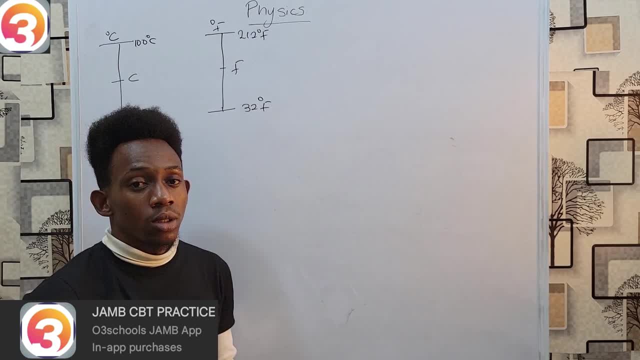 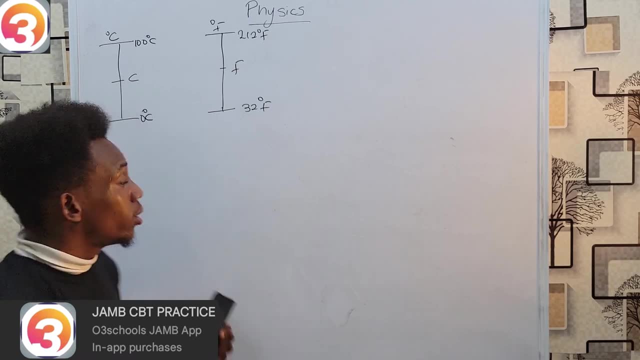 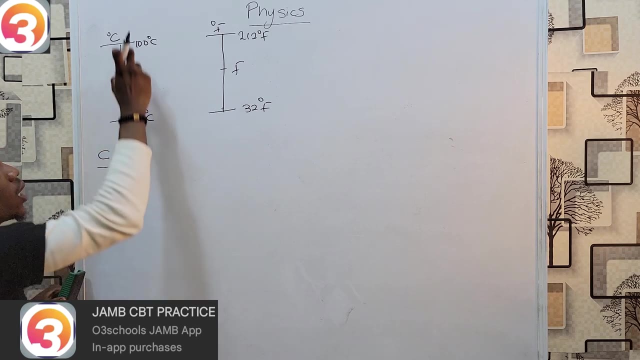 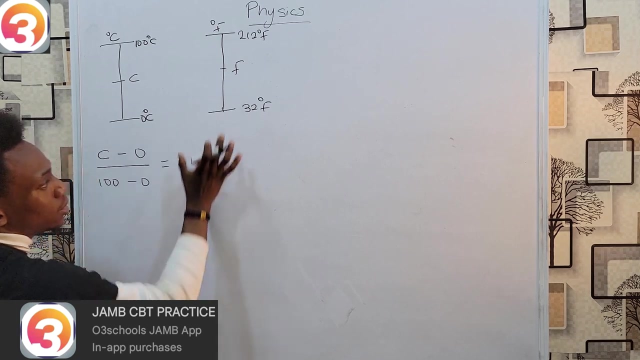 now we apply a simple method known as interpolation. what you simply do is you shall be working on the fact that these things should have fixed differences or fixed increase. therefore, taking your middle value c minus the bottom value, zero over the top, 100 minus zero equals. and now you repeat the exact same thing on the right side: middle value again, f minus bottom. 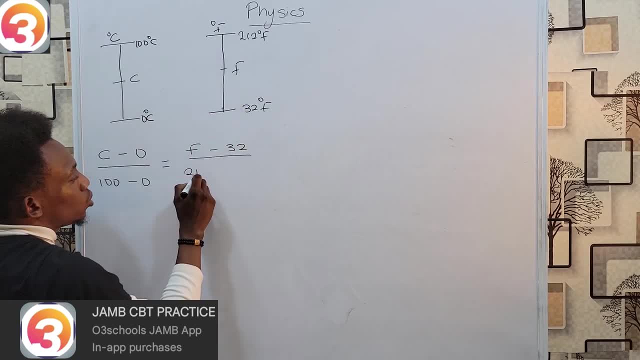 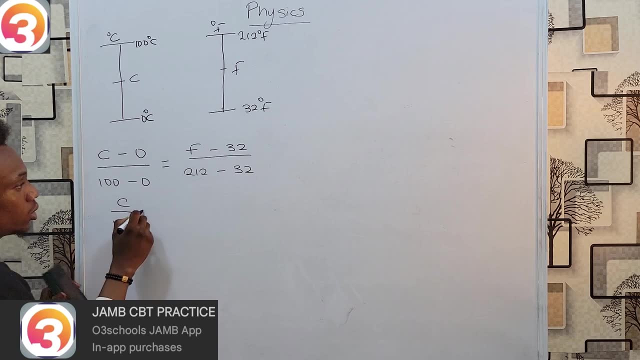 32, all over top. 212 minus 32. c minus zero is c, 100 minus zero is 100, and this is f minus 32, and 212 minus 32 is 180.. so from here, simple arithmetic: zero can count to zero. two into ten is five, into eighteen is nine. first, multiply nine c. 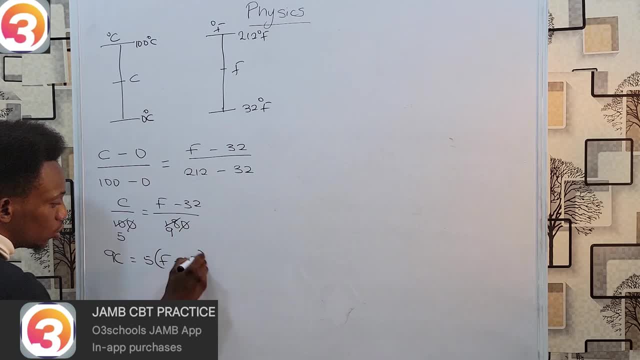 plus five into f minus 32, and if i have to get this over nine, over nine, so the value in celsius can be gotten by saying five over nine minus f minus 32.. and so you can see, this gives me my value in celsius when i know my value in fahrenheit. now some of you might already be saying: 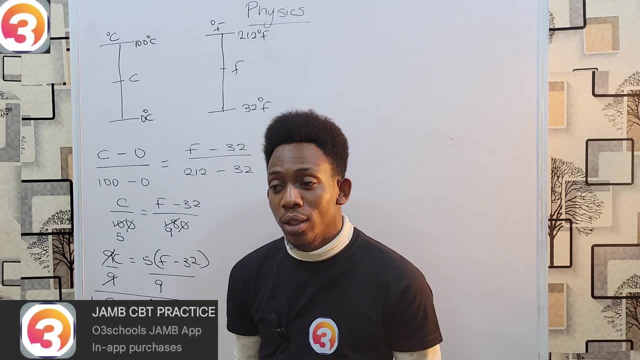 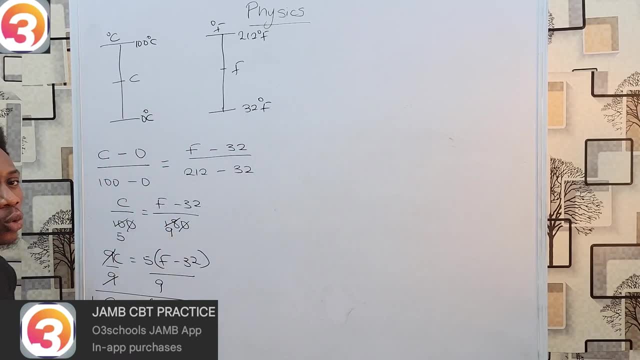 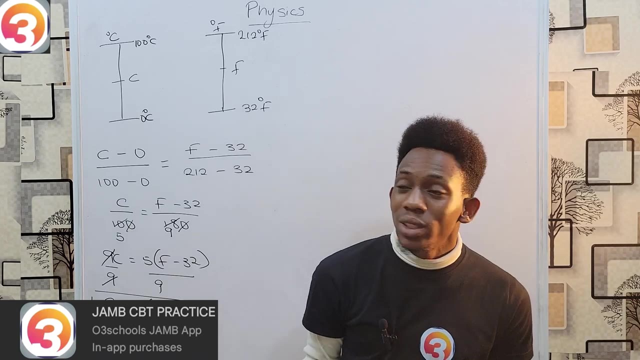 how can i memorize formulas, each and every single one? well, please you to know, you only have to memorize formulas when you are dealing with kelvin, because that formula is quite simple, pure addition for every other question. you do not memorize the formulas, rather, you go through certain steps, like we just went through and solved. 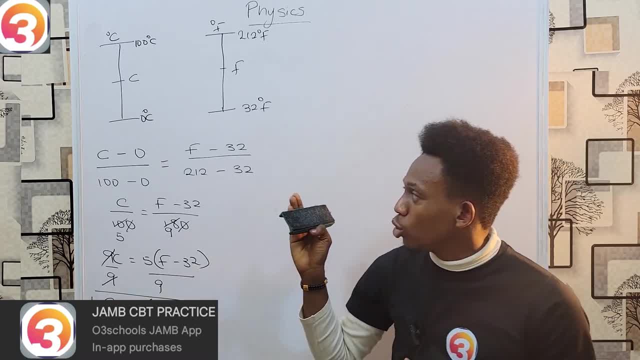 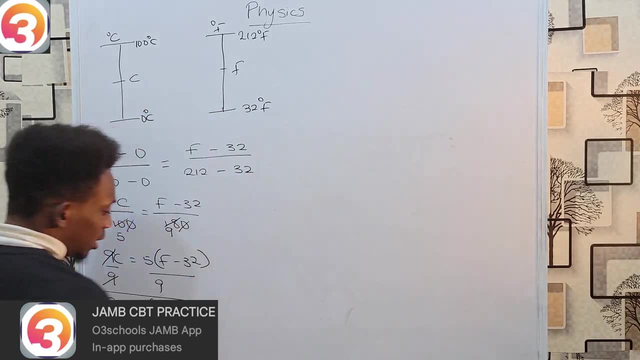 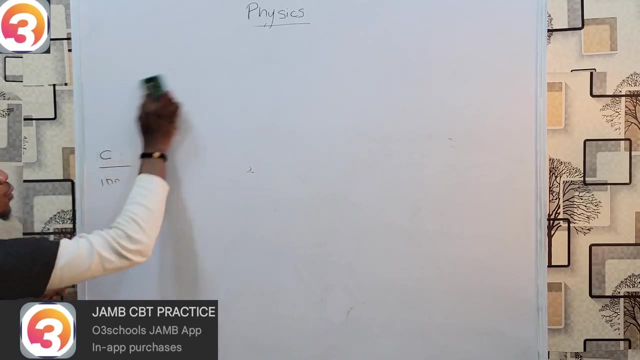 them individually, always top, bottom. then you simply say middle minus bottom over, top minus bottom. and if this conversion method is understood, it is time for us to take a few examples, which, of course, we shall be doing using the aids of our old three schools. jump app question search. 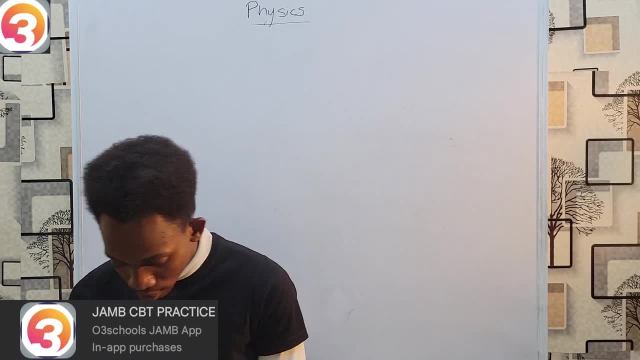 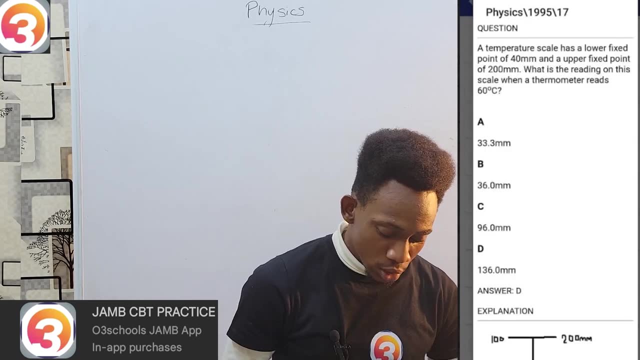 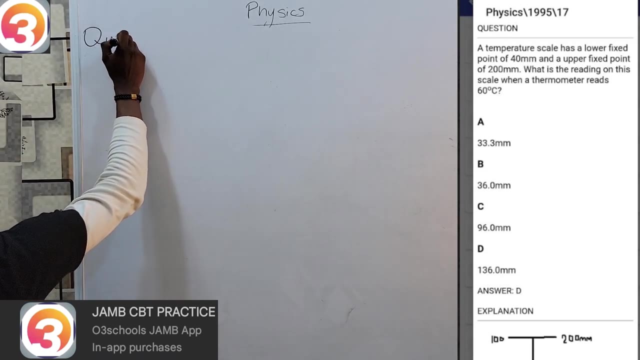 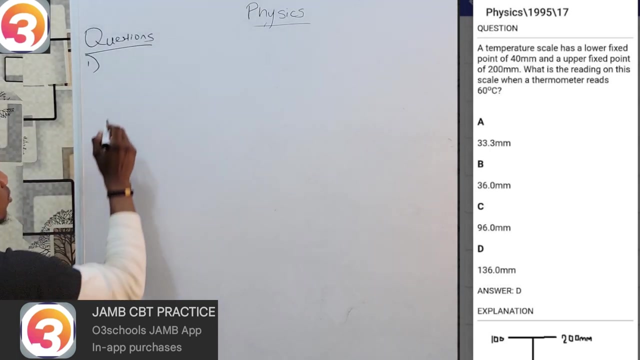 so if i also go to my old risk with jump app and um, yeah, question already the year 1995, question 17.. this question says a temperature skill. i've got questions now. a temperature skill has a lower fist point of 40, which means if i draw this right now the lower fist point is 40 millimeters. 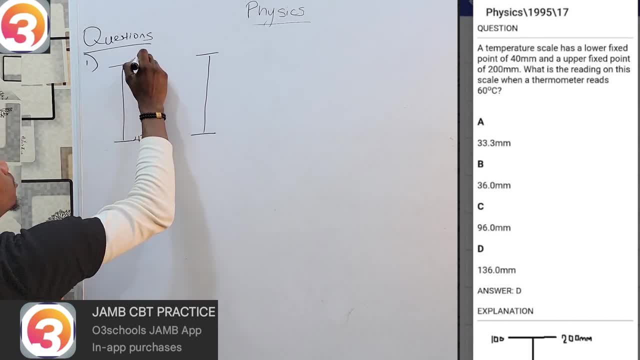 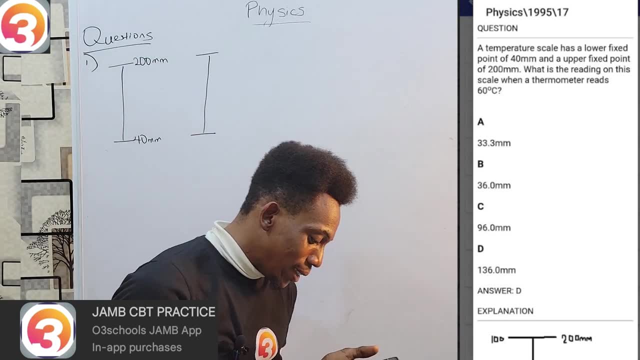 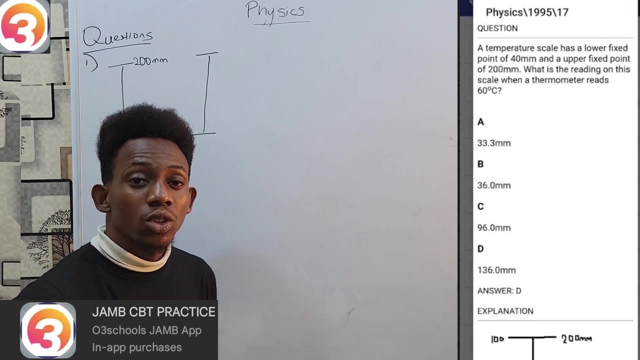 and upper fist points of 200 millimeters. okay, what is the reading on this skill? a thermometer reads 60 degrees celsius, because they're asking me about something. degrees celsius, that must mean that the next thing i'll draw is 100 degrees celsius and zero degrees celsius. 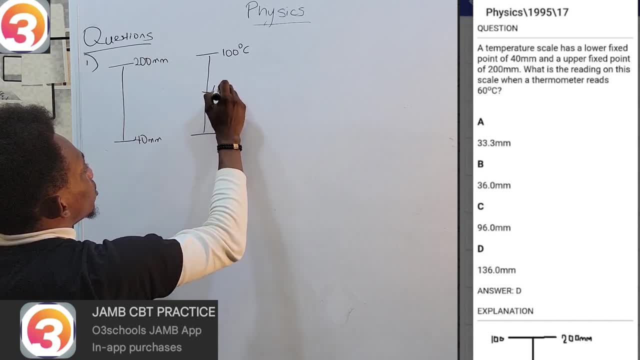 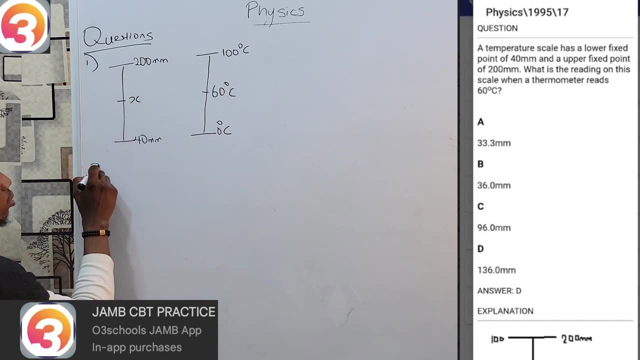 so what is the reading? when this torment, i show me 60 degrees celsius. i can call this x. then, using a method that's outside previously, middle x minus bottom, 40. e over top 200 minus bottom. also, 40 equals middle 60 minus bottom. zero over top 100 minus bottom. 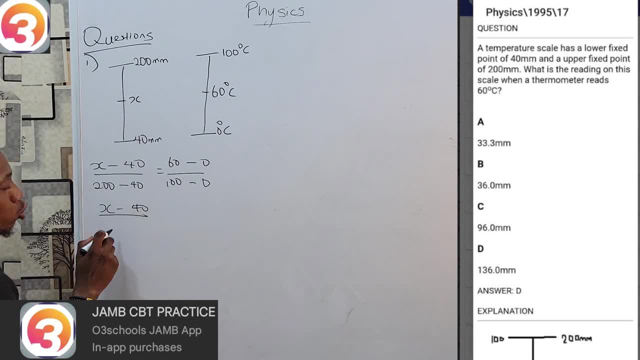 zero. so x minus 40 over 200 minus 40 is going to be 160 plus two. sixty minus zero. sixty hundred minus zero one hundred. so let's see what can cancel out zero. to scale zero to x, care of zero. so if i cross, multiply x minus 40 times, one obviously is minus 40. 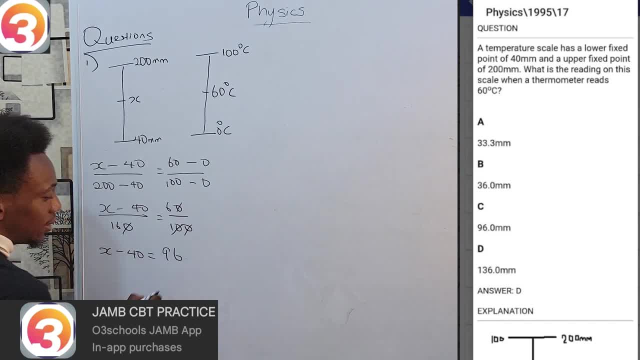 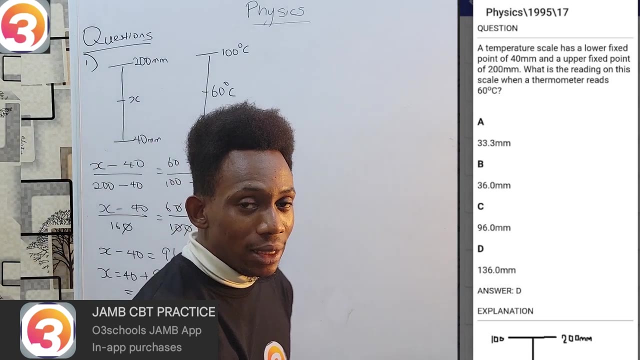 then 16 times 6 will be 96.. so x equals to 40 plus 96, which gives 136 millimeters, and obviously that is my option d. as you can see, these questions are quite simple. just note to me that these are the equations that are the answers that are often used to determine whether or not we have middle and lower fist points. 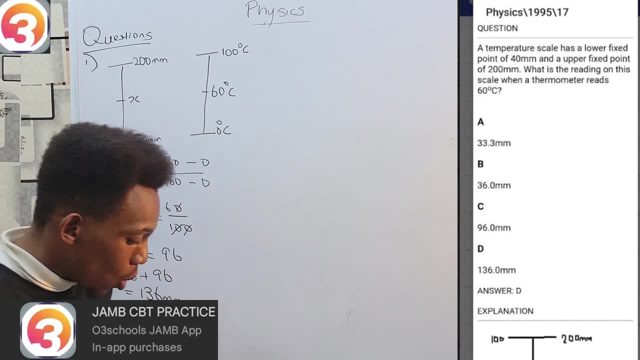 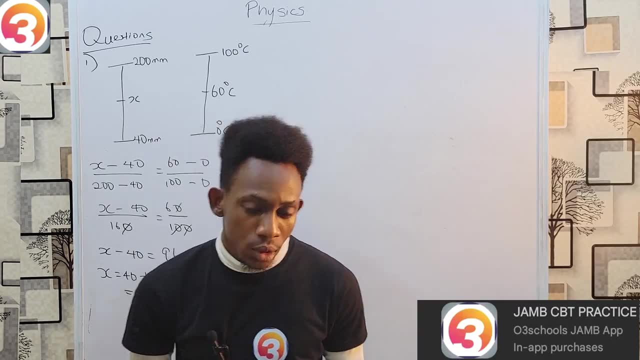 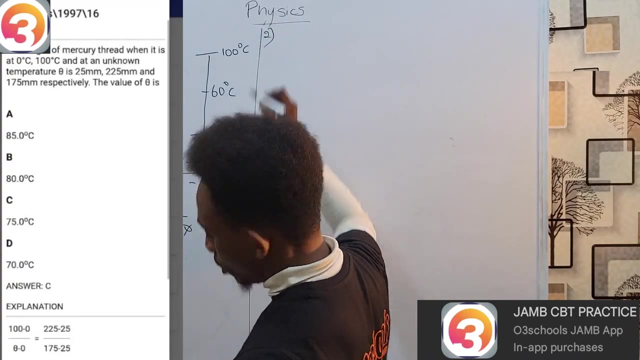 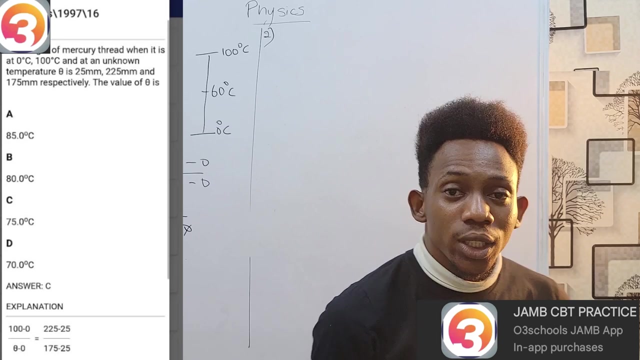 just notes the upper and the lower fist points. okay, trying another, we shall go to the 1997. I shall look at question number 16. the year is 97. the question is 16: the length of mercury trade when it is at zero degrees Celsius hundred. 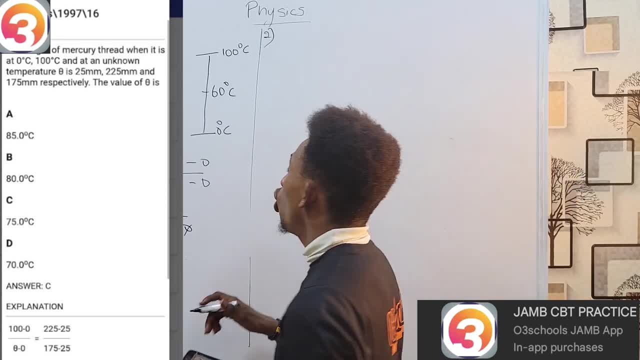 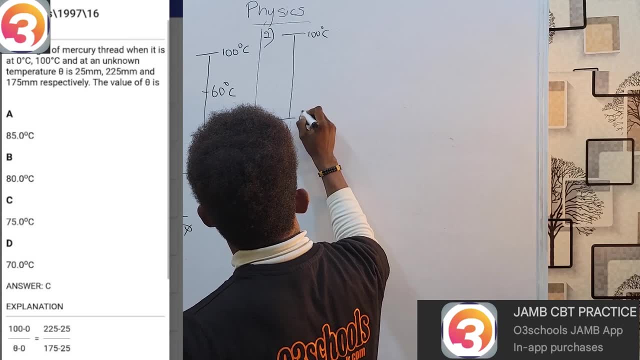 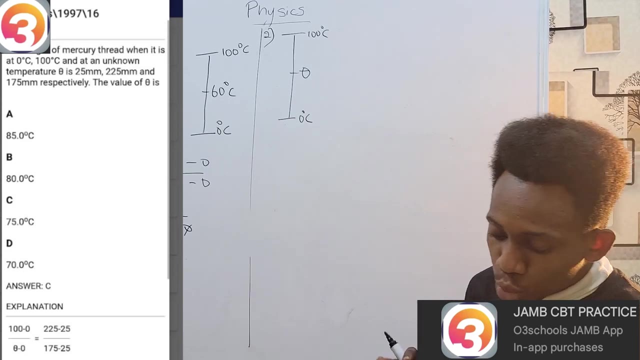 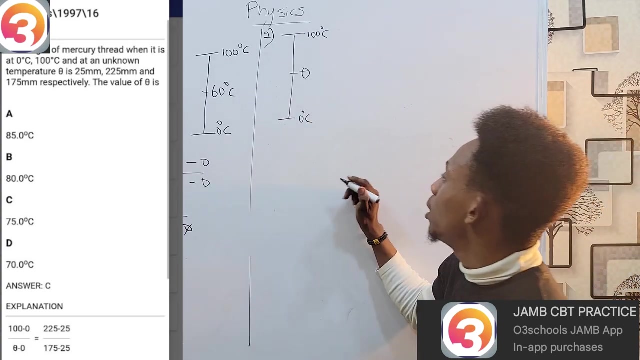 degrees Celsius and an unknown temperature, automatically. I know that my best Coulomb was being Celsius, hundred zero and unknown temperature. theta is 25 millimeters, two to five millimeters and 175 millimeters respectively. so if I draw my second, I know that respectively implies that the first thing they told 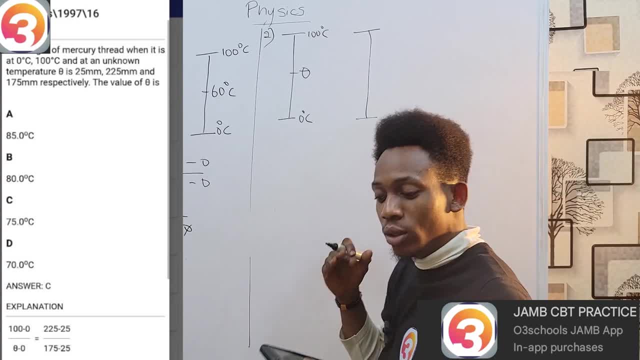 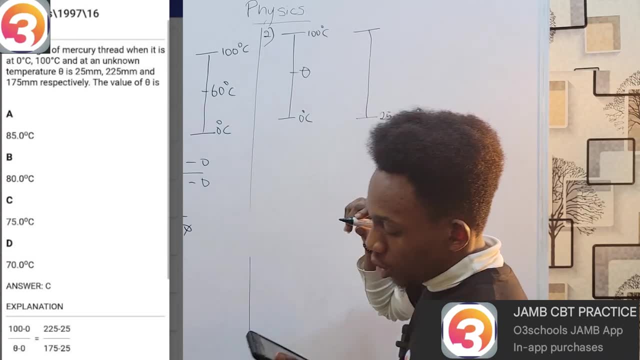 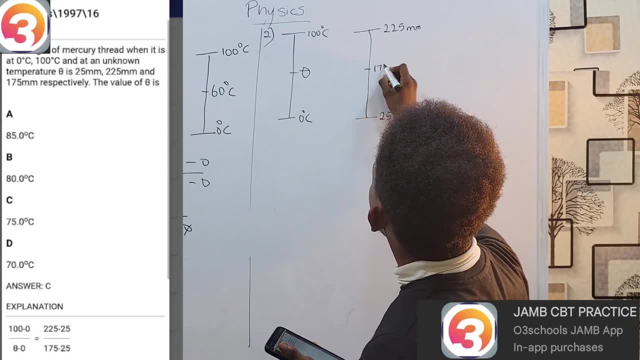 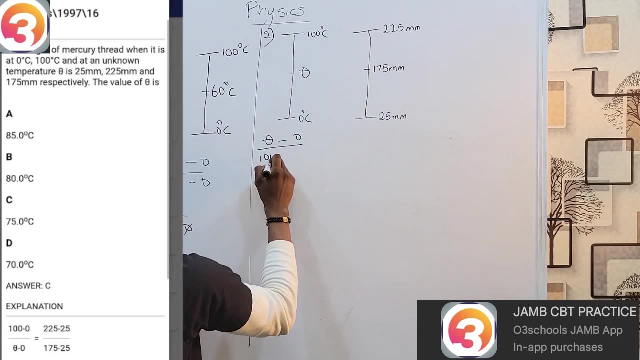 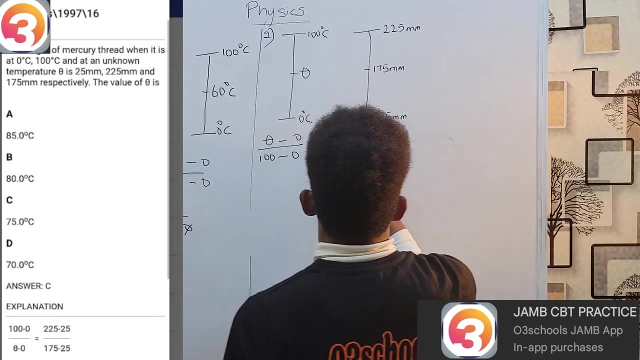 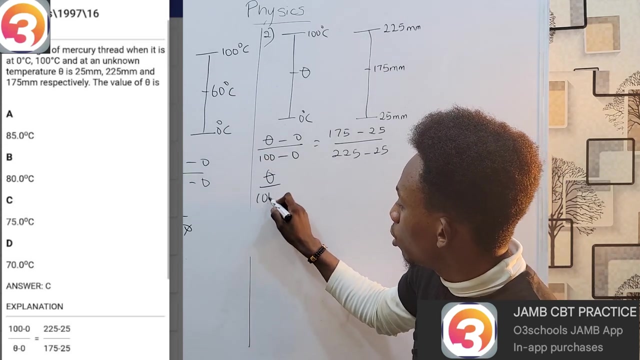 last but not least, theta is 175 millimeters, implying that this week t-minus zero, about hundred minus zero, was still 175 minus 25 over two to five minus 25 five. so t-minus zero is tita, hundred minus zero is hundred, 175 minus 25 is. 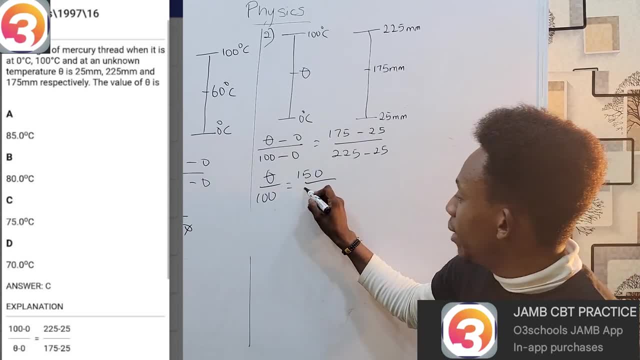 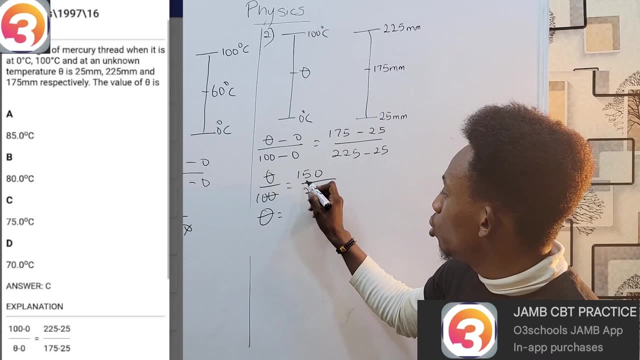 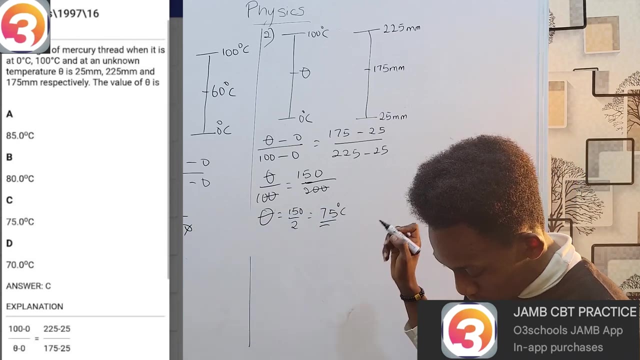 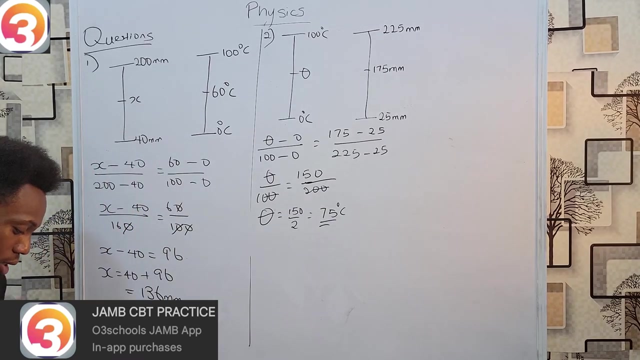 one fifty two to five minus 25 is 200, but my zeros cancel these two zeros. Tita equals 250, over to which will be 75 decrease Celsius. that is my option. see I, this is quite simple. keep the basic idea in mind, draw your lines and you pretty much have your answer. trying one more. 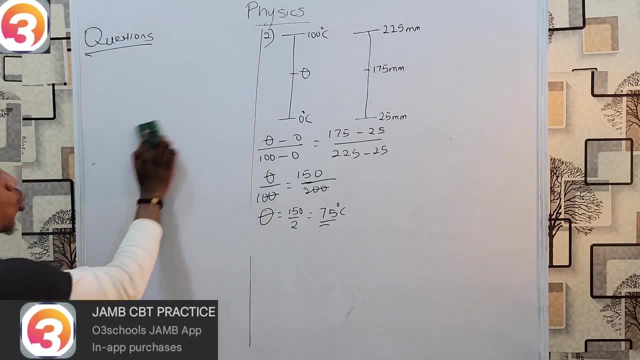 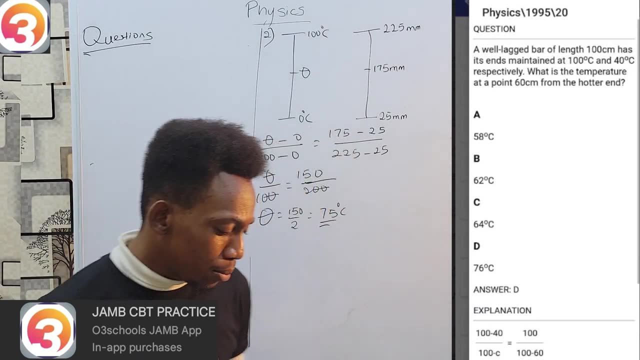 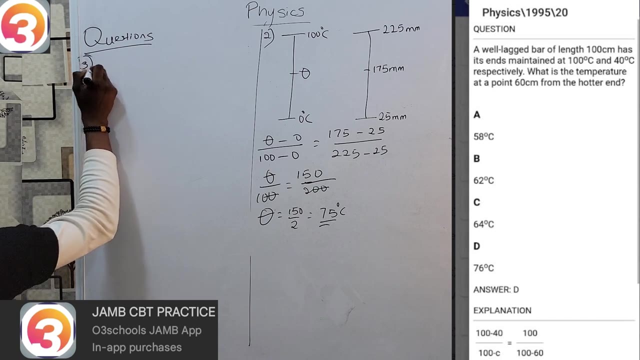 this is from 1995 and this is question number 20. a well-lagged bar. do not say the way it's deceiving you. a lagged bar simply indicates a well insulated bar. now, this bar has a length of 100 centimeters and the ends are maintained at 100 degrees celsius and 40 degrees celsius. 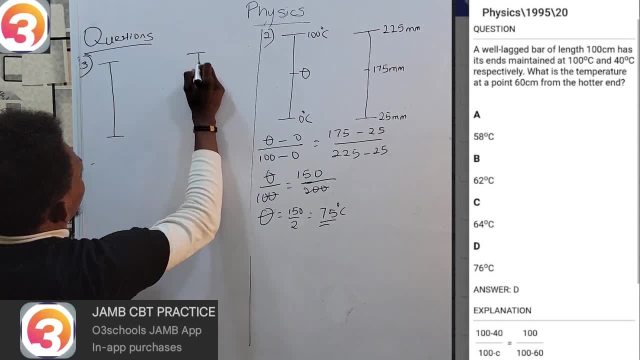 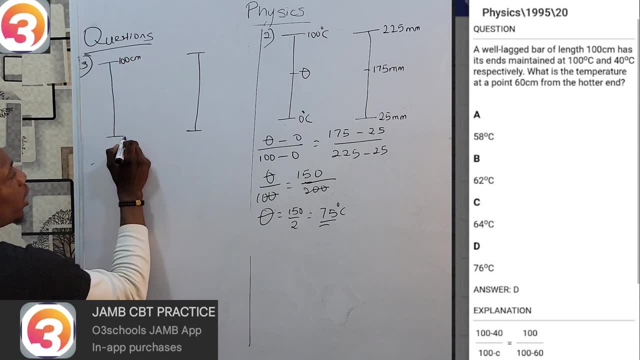 so if i'm going to draw my columns now, first i say, okay, how do we do this one? i have a bar 100 cm. if i call you, 100 cm of the bar here is zero cm, which has to start somewhere and end at 100. 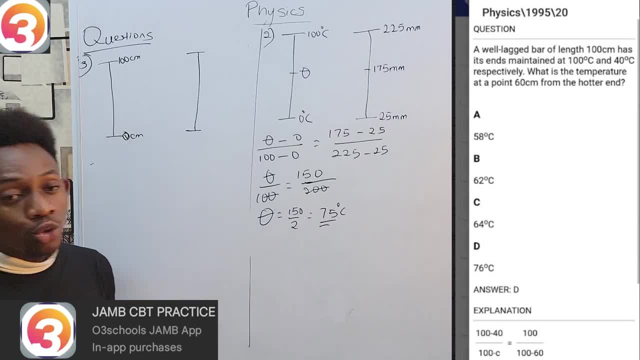 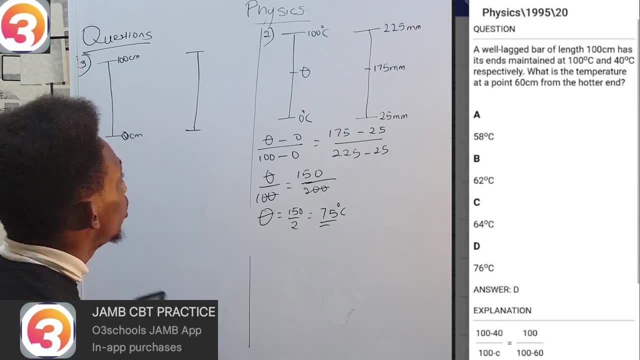 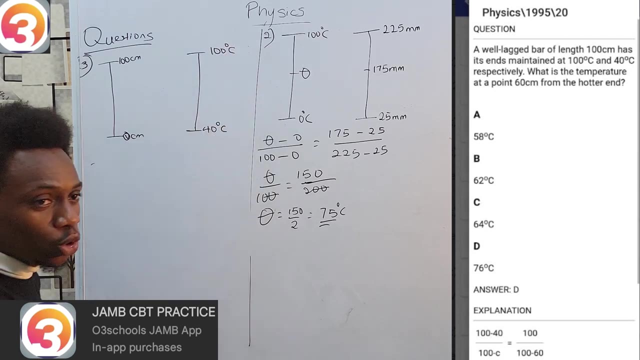 now i'm told that these ends are maintained at 100 degrees celsius and 40 degrees celsius. those are my ends. there's no space for which end should be which, so i could decide to put my 100 degrees celsius up here and my 40 degrees celsius down there, switching it around to achieve the same. 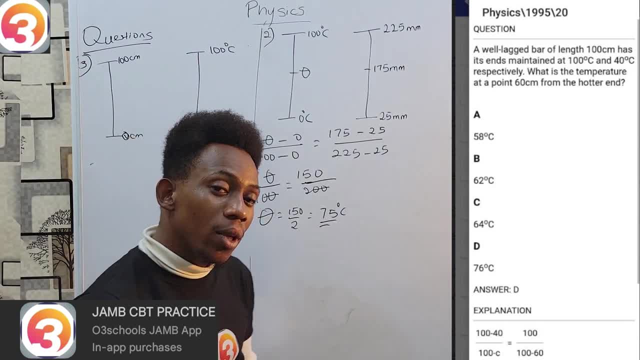 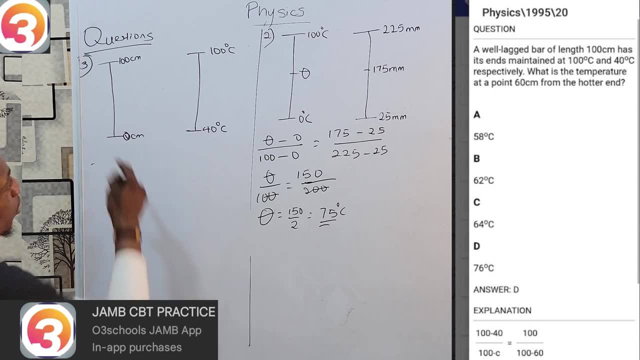 results. what is the temperature 60 cm away from the hotter end temperature at the point 60 cm from the hotter end? now, based on my current arrangements, my hotter end 100 of my 100 cm mark. now i'm meant to go 60 cm away from that 100 cm mark. so if i'm to go 60 away from 100, 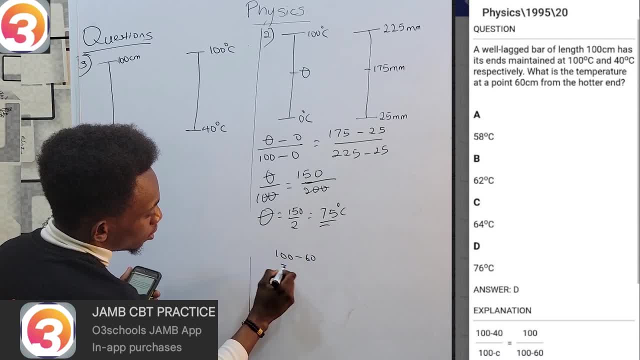 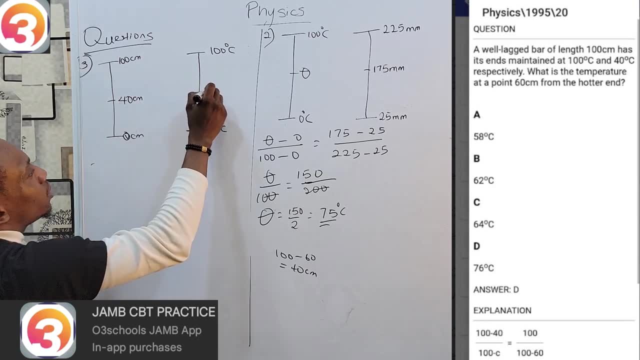 that will be going down here: 100 minus 60, which is 40 cm, which means that, truly, i am at my 40 cm mark and i want to find the temperature, which we shall call x. so from here, the same method that we've been using since my middle: 40 minus bottom. 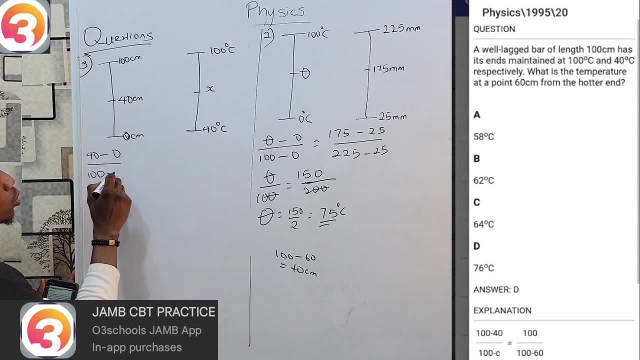 zero over top hundred minus bottom zero. middle x minus bottom 40 over 100 minus bottom 40. 40 minus 0 is 40. 100 minus 0 is 100 x minus 40 over 0 minus 40 is also 60. so let's see: 0 cancels 0. 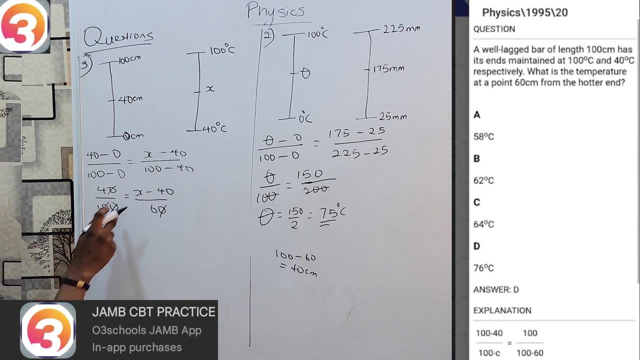 0 also cancels 0. therefore, x minus 40 times 1, x minus 40 4 times 6 is 24.. so x will be 24 plus 40, indicating that x is 64 degrees celsius. so temperature day is 64, which is: 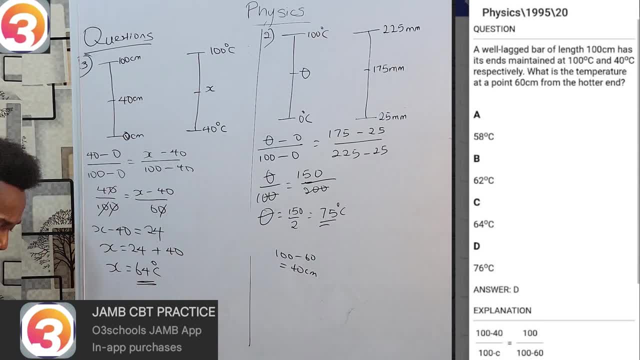 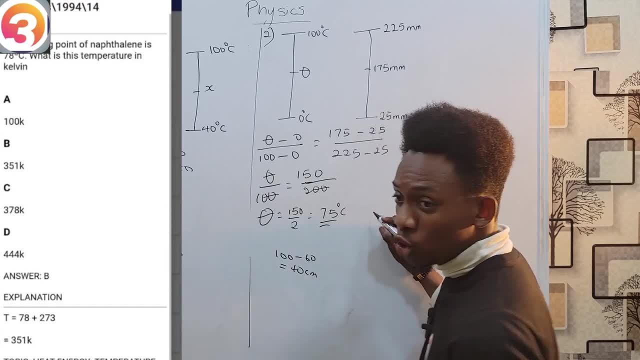 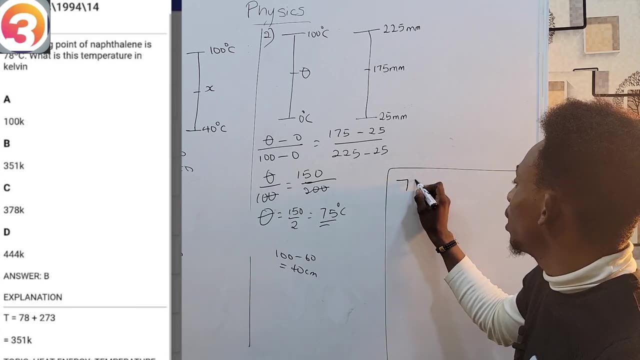 option c. so you see, these are quite rudimentary. um, there's a simple one which will take us up to two lines, so i'll simply just do it right here. we have been told the melting point of naphthalene is 78 degrees celsius. and the melting point of naphthalene is 78 degrees celsius. 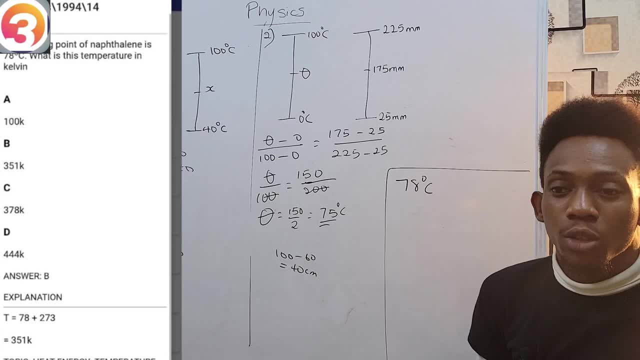 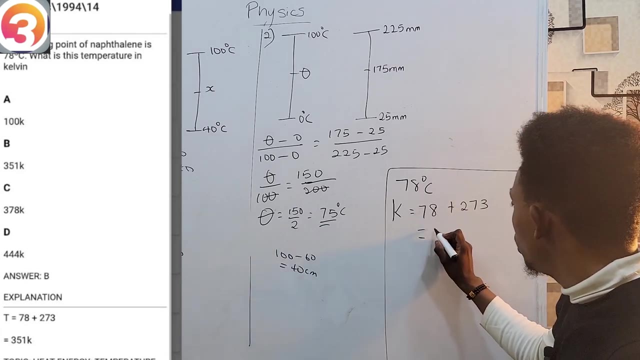 and the melting point of naphthalene is 78 degrees celsius. was this temperature in kelvin? like we said, when we go from kim to celsius, something becomes very simple. simply add 273, so 273 plus 78 presents your calculator. you should be getting 351. 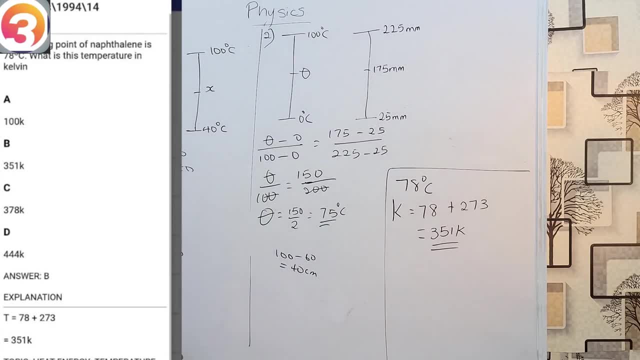 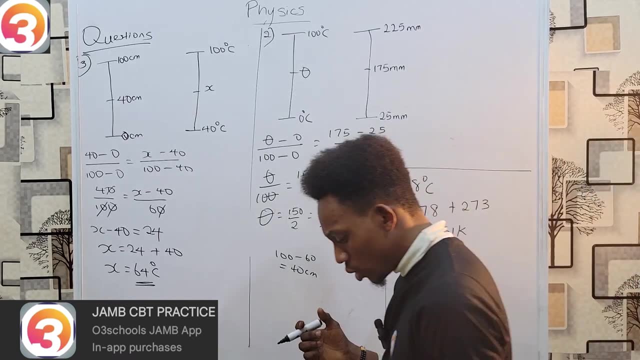 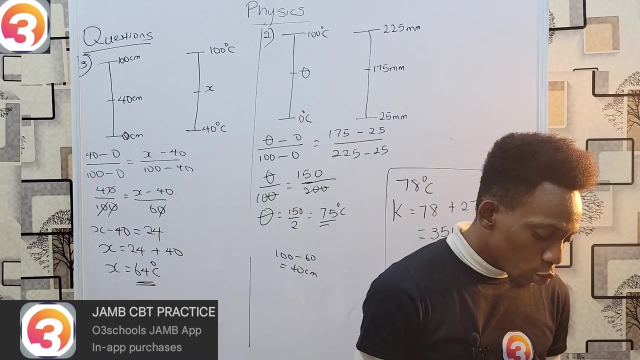 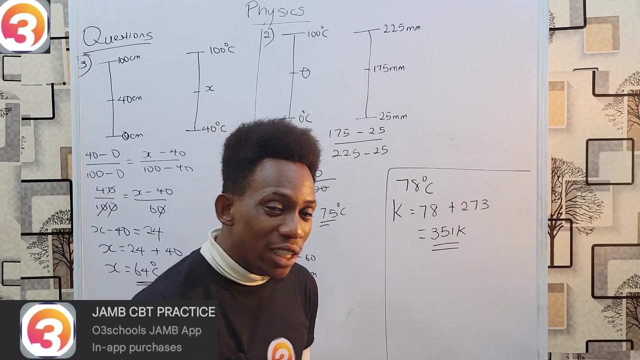 kelvin. and so you see, these steps are quite, quite simple. um, okay, now we have a theoretical question to answer. this one says the thermometer who's reading is indicated by a change in color of its metric property. by the way, this 2009 question 18.. so meter whose reading is indicated? 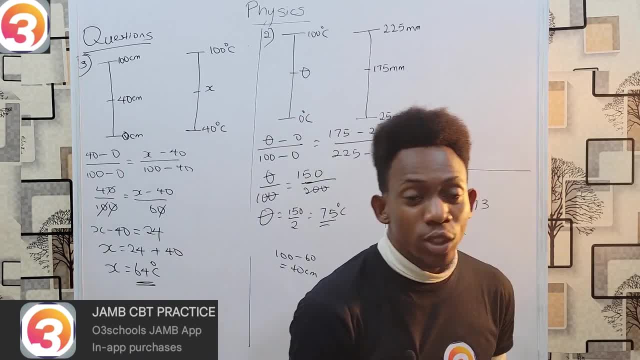 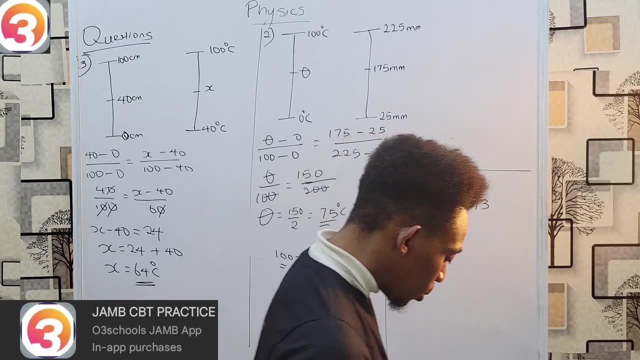 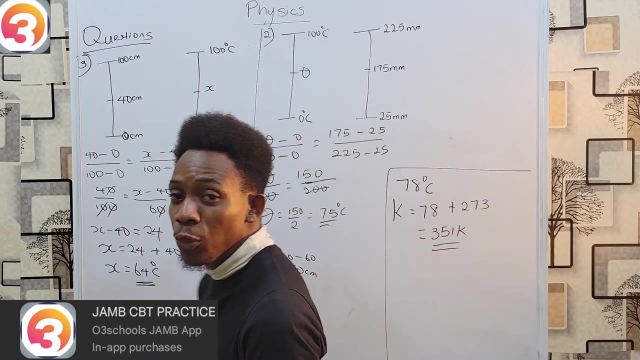 by change in color. well, the rough chunks are dialectic strip, thermometer, thermocouple, resistance thermometer and optical parameter. even without any knowledge, we are seeing there's a change in color. you observe a change in color with your eyes, and what does that have to do with optics? so 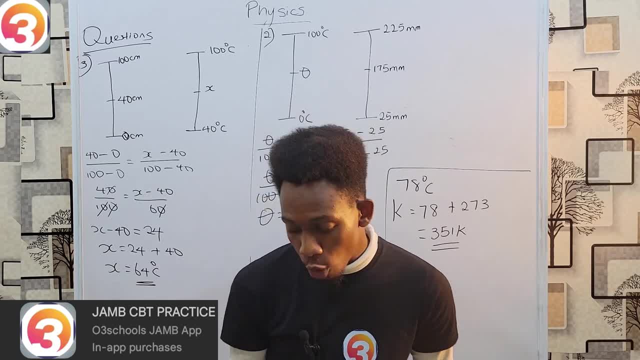 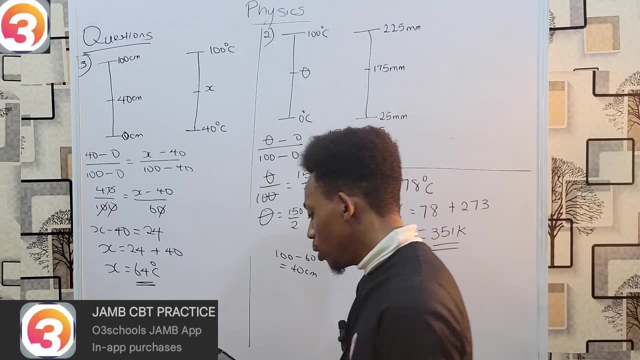 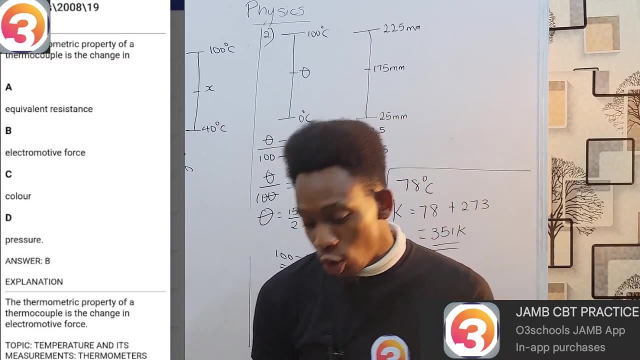 instantly, I should be able to tell my answer is the optical parameter. see, so these are just very, very simple. we also have the thermometric property of a thermocouple is the change in watts. we looked at this at the beginning of the class change in watts for thermocouple with valiant resistance. we said no resistance as 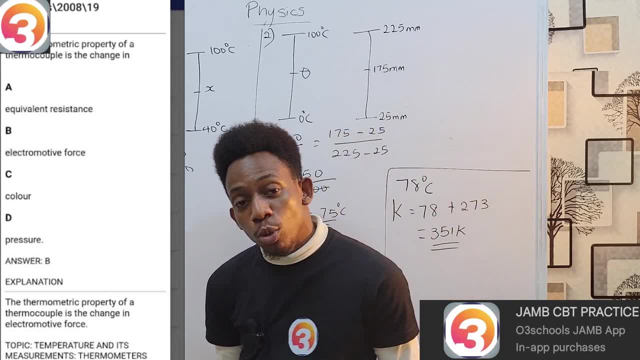 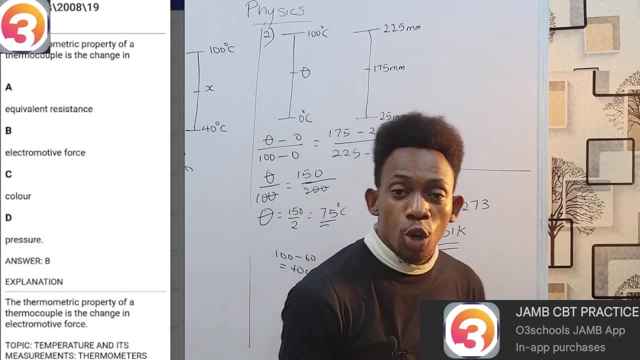 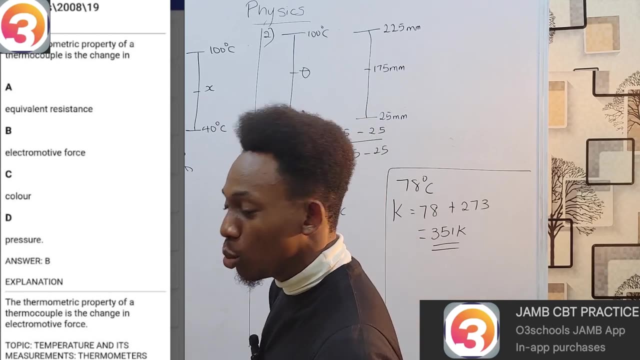 with the resistance thermometer, obviously? well, there's electromotive force sign. well, yes, that is my answer. we should also analyze the other options. color: I could just say it works for your optical parameter. white pressure is for your gas thermometer. so my answer is electromotive force, option B, and this was from 2008. 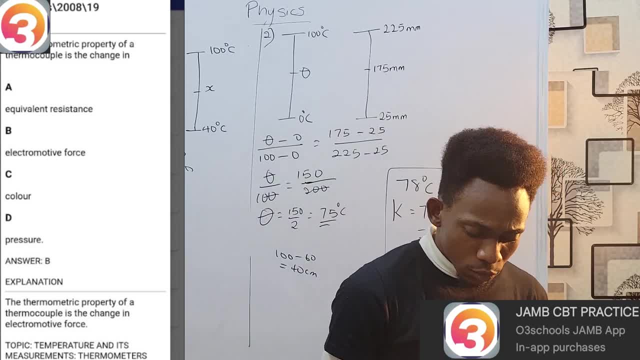 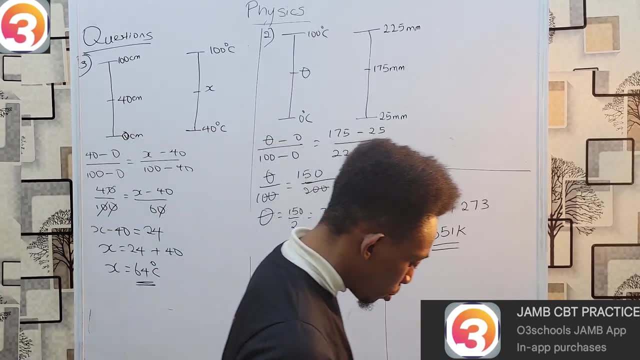 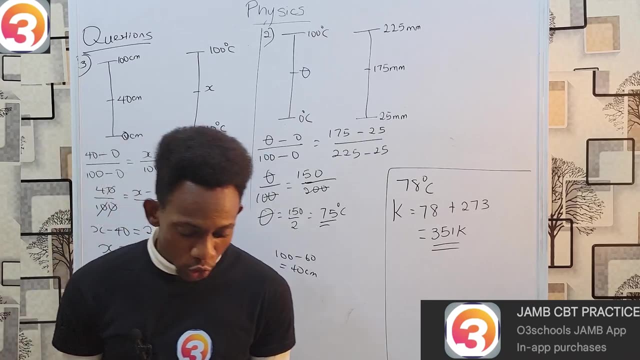 question number 19 JC. there are many other questions you shall find on this topic. when you try to solve them, you shall use the exact same method as we've been using so far and you shall get your answers like: okay, let's try some more theoretical questions. shall we? water is a? 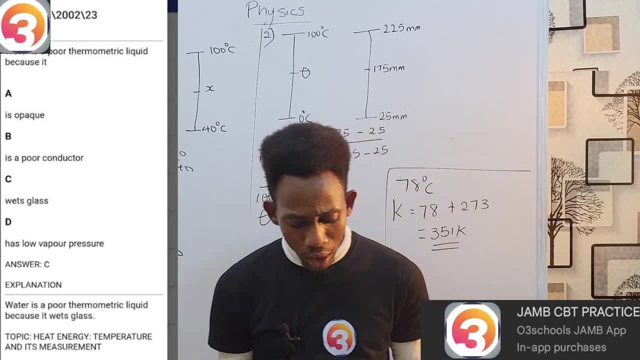 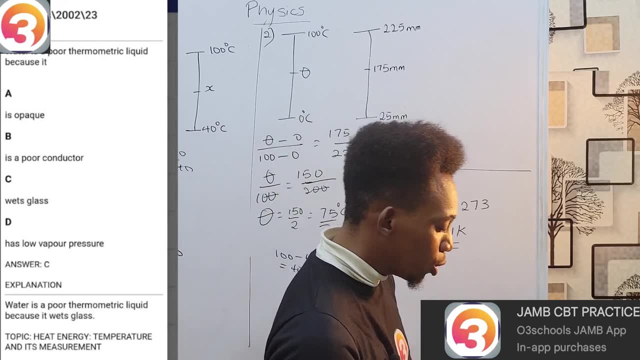 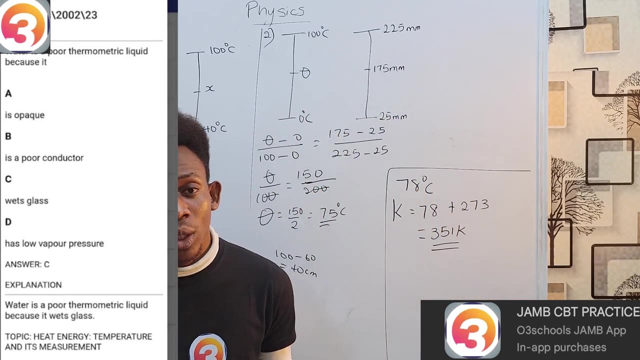 poor thermometric liquid because it's watts. again, we've answered this during our explanation. this one is from 2002. question 23: why is water a poor thermometric liquid? option A: they said it is opaque and whether there is no people today's transparent you are see through water it.